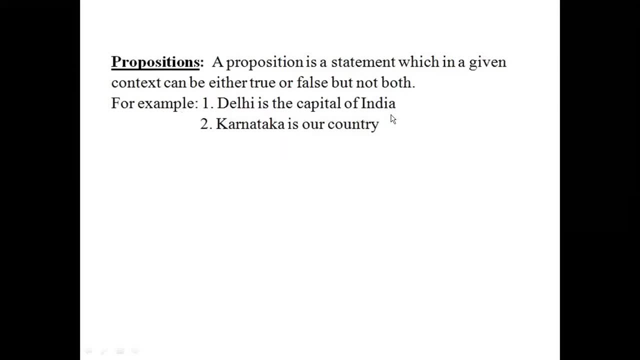 Delhi is the capital of India is a true statement. Secondly, another example I have taken: Karnataka is our country, which is a false statement. So propositions are nothing but the statements, which helps us to know whether, in the given context, the statement is a true or a false. 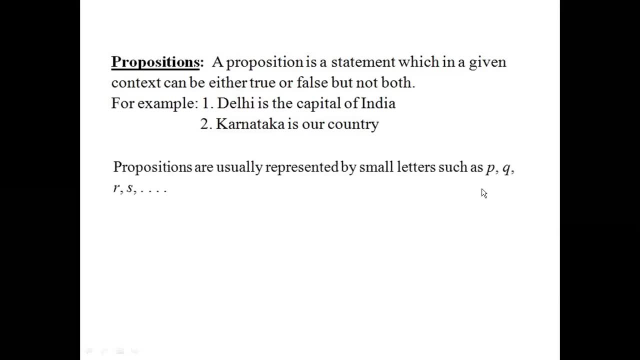 Propositions are usually represented by small letters such as P, Q, R, S, etc. The truth or falsity of a proposition is called its truth value. So either the statement will be a true or it will be a false. So the truth or the falsity of such a statement or a proposition is known as its truth value. 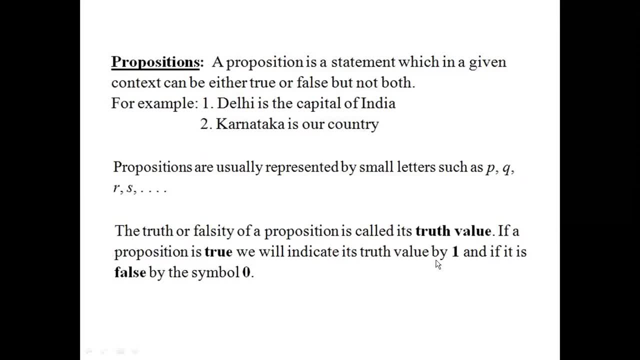 If a proposition is true, We will indicate that it is true. We will indicate its truth value by 1.. If the proposition is false, then we use the symbol 0.. So while writing the truth tables, we assume either zeros or ones based on the proposition. 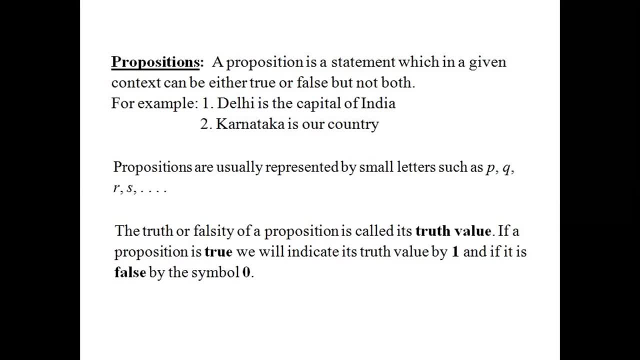 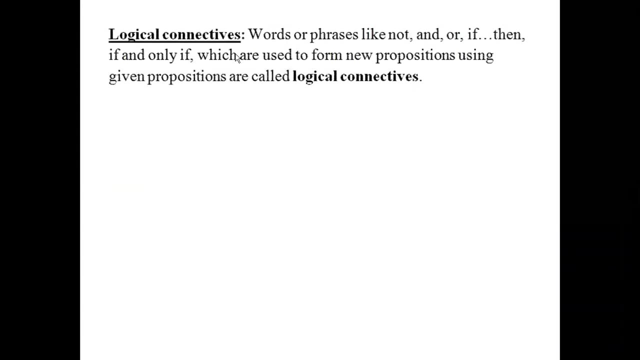 statement, whether it is true or false. So we assign 1 for a truth value and we assign 0 for a false statement. We will understand about logical connectives, Words or phrases like NOT, AND OR, IF, THEN, IF & ONLY IF, which are used to form new propositions. 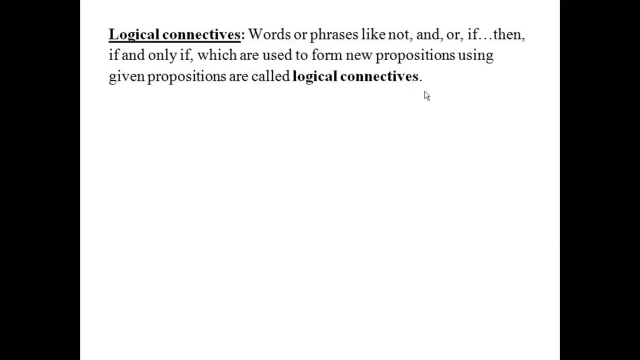 using given propositions are called logical connectives. So suppose we wish to combine two statements And we would use some of them. Some of these connectives like NOT AND OR IF, THEN, IF & ONLY IF, etc. Then such propositions using these connectives are called as logical connectives. 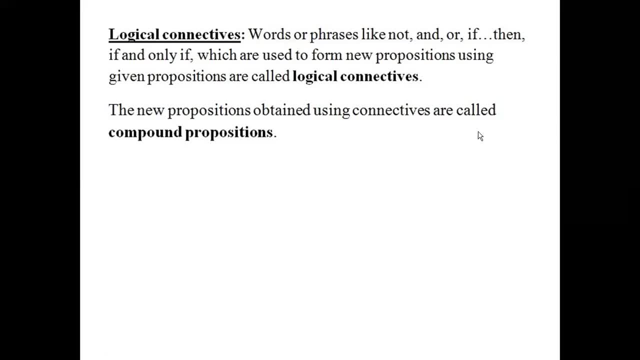 The new propositions obtained using connectives are called compound propositions. So, using the connectives, whatever the new propositions we obtain, they are known as compound propositions. The original propositions from which a compound proposition is obtained are called the primitives or the components of the compound proposition. 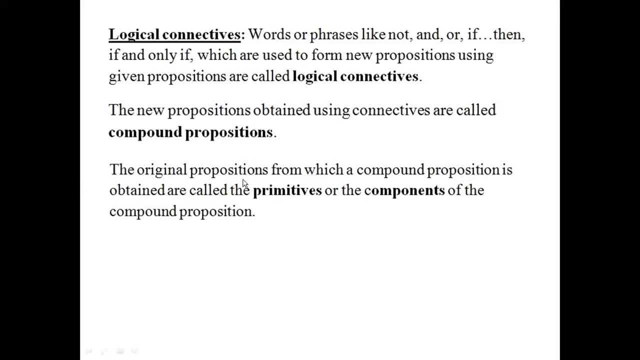 So the original propositions we have used, from which, using the logical connectives, we obtain a compound proposition. So, whatever the original propositions are there, We use them or we call them as primitives or the components of the compound proposition. Propositions which do not contain any logical connectives are called simple propositions. 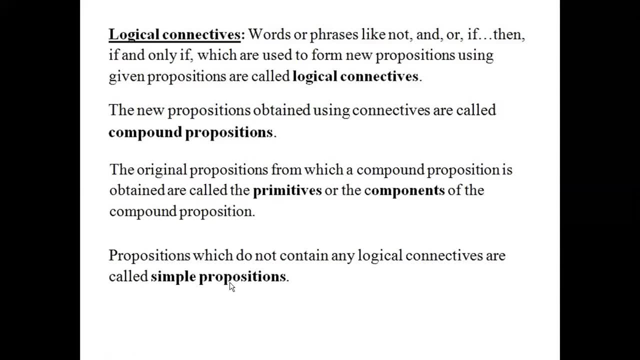 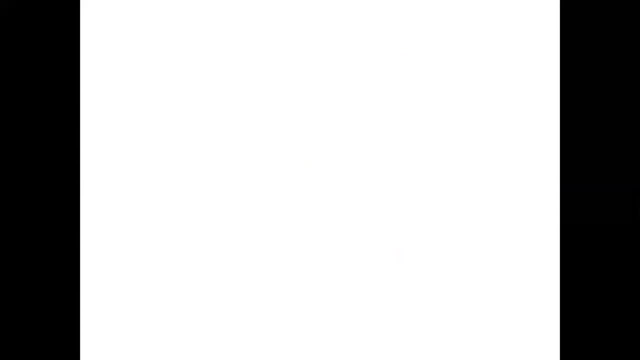 It is usually a proposition without any logical connective is known as simple proposition. So if you use the logical connectives like AND, OR, IF, THEN, etc. Then such propositions are compound propositions. Next we will learn about negation, A proposition or that. this is also a statement obtained by inserting the word NOT at an appropriate. 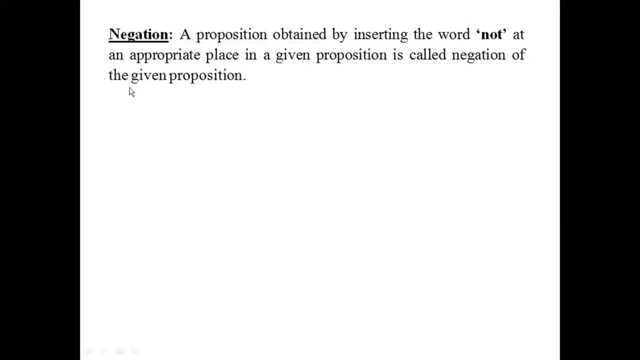 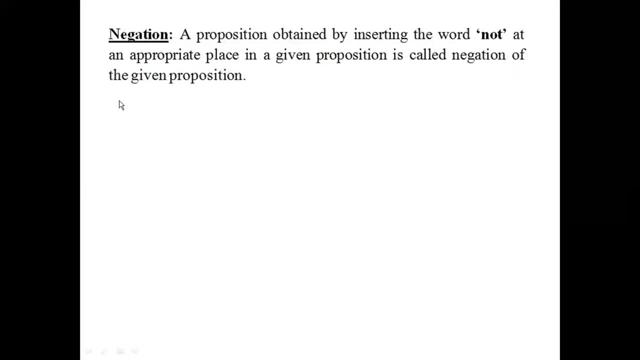 place, then we are using the negation. we are obtaining the negation of the given proposition. The negation of a proposition P is usually denoted by the symbol. We call this as tilde tilde P. It is usually read as NOT P. 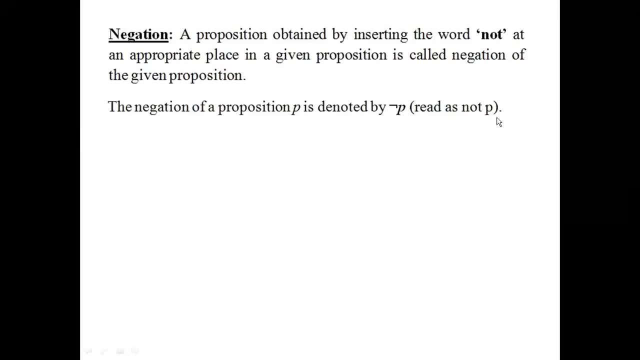 Negation of P or NOT P Conjunction: A compound proposition obtained by combining two given propositions by inserting the word AND between them, is called a conjunction of the given propositions. So conjunction stands for the symbol, AND If you want to combine two given propositions using the symbol AND then you can use the, 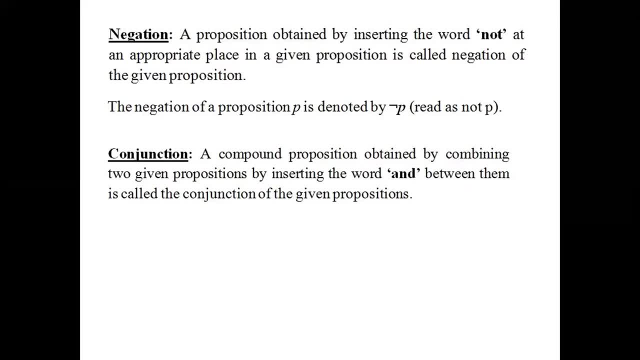 cmd key. If you want to combine two given portions using the word AND, then the resultant will be the conjunction of the given propositions. So to terrible it is. The conjunction of P and Q is usually denoted by P AND Q. The symbol is reverse V. 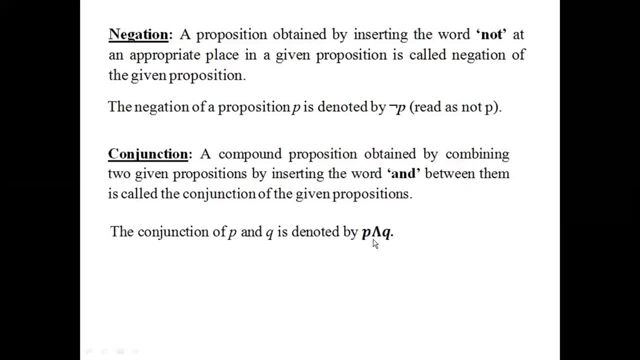 The sideways position of reverse V is the symbol used for conjunction or AND. The square position of V is always used for conjunction. The square position of V is the worst one. So square position of the negative, positive here is J. So square position of the negative, negative here is J. 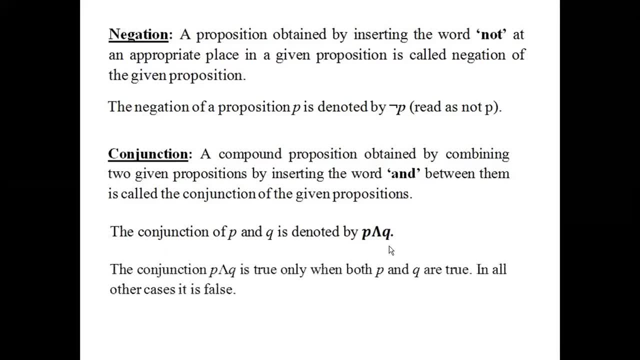 We say we must use only the verb and whatever the whom, So Dragon styles can be used for conjunction with an end, conjunction that adds, or a remark on a negative word which is outward ground. That is when we use the verb as the only future conjunction in a sentence, but only on a condition. 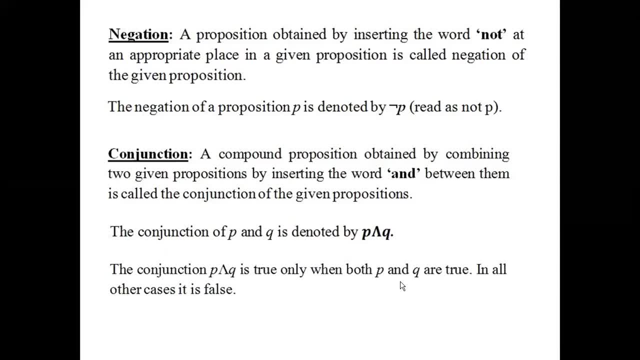 Q is true only when both P and Q are true. In all other cases it is false. So it becomes very important to know about these definitions to form the truth tables. So when will P and Q be true? The truth value will be 1 only when both P and Q have the truth value 1.. 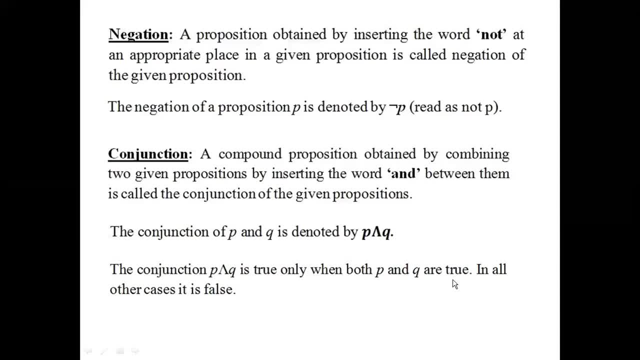 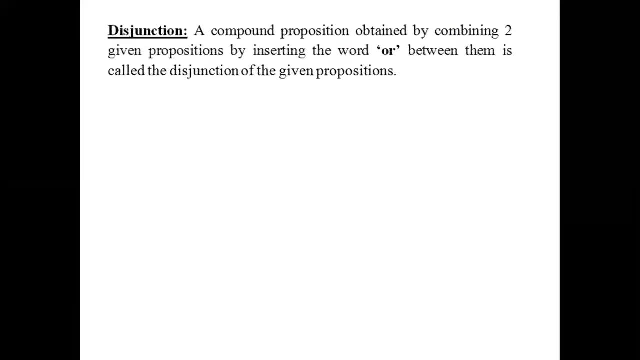 That is, only when both P and Q are true, we have the truth value of P and Q to be 1.. In all other cases, the truth value will be 0.. Next definition is about disjunction: A compound proposition obtained by combining. 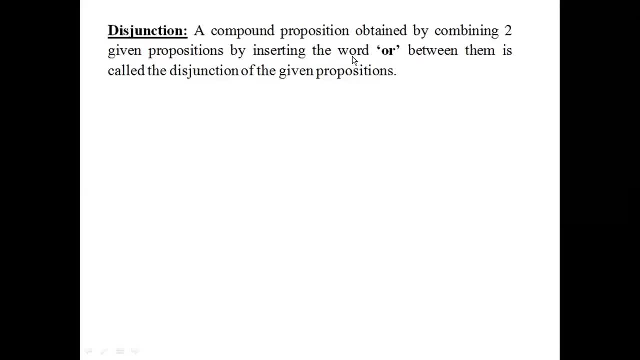 two given propositions by inserting the word or between them is called the disjunction of the given propositions. So suppose, given two statements, we want to use the word, or then the resultant would be the disjunction of the given statements. So the disjunction of P and Q is usually denoted by P or Q. In the middle we have a V symbol. 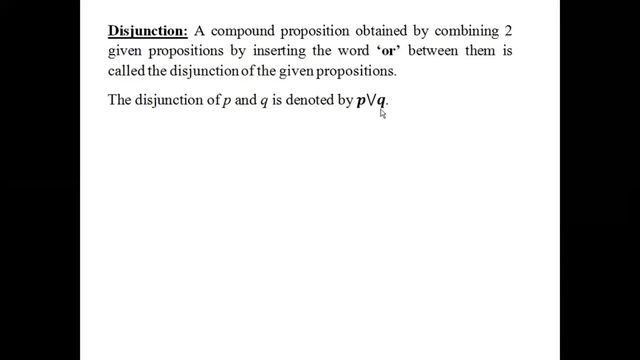 So P or Q represents the disjunction, And the disjunction P or Q is false only when both P and Q are false. In all other cases it is true. So P or Q has the truth value 0 only when both P and 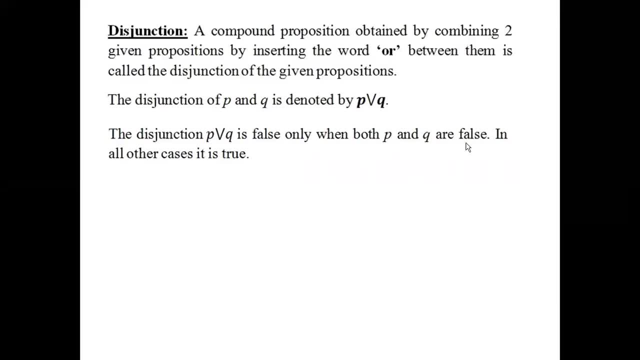 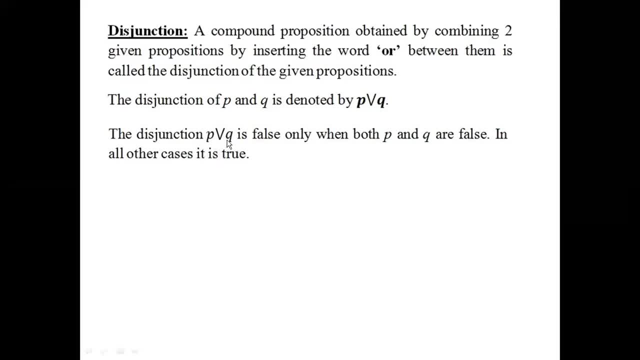 In all other cases, the truth value of P or Q is false. In all other cases, the truth value of P or Q is false. In all other cases, the truth value of P or Q is false. In all other cases, the truth value of P or Q is true. 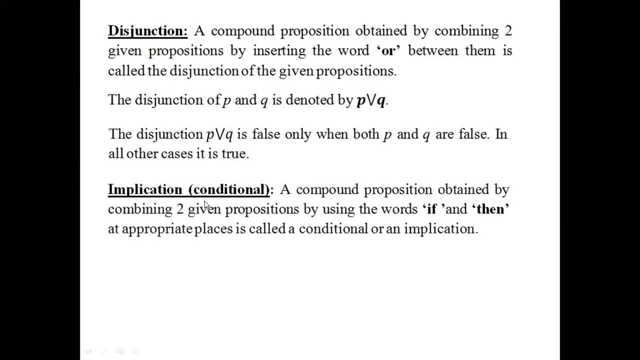 Next we will learn about implication or conditioning. A compound proposition obtained by combining two given propositions by using the words if and then at appropriate places, is called a condition, conditional or an implication. So we have a given compound proposition, We obtain a. 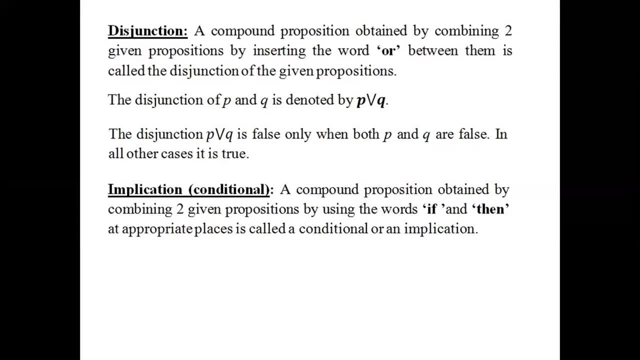 compound proposition by combining two simple propositions using the given words like if and then at appropriate places, Then the resultant would be the application of conditional or an implication. If P, then Q is denoted by P, a right arrow Q. But we read this while doing: 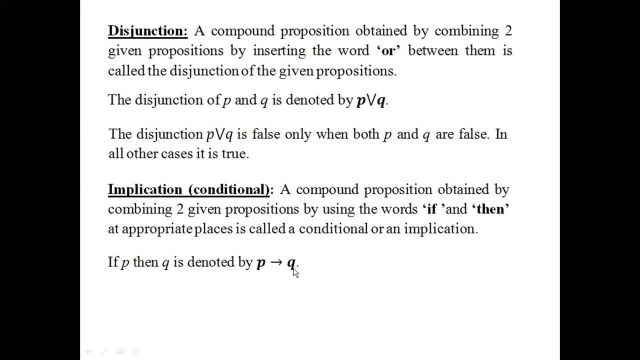 problems as P conditional Q or P implication Q. We can also read it as if P then Q. The conditional is false, P conditional Q or P implication Q is false only when P is true and Q is false In all other cases. this is true. So this is the rule, what we apply in implication or the conditional. 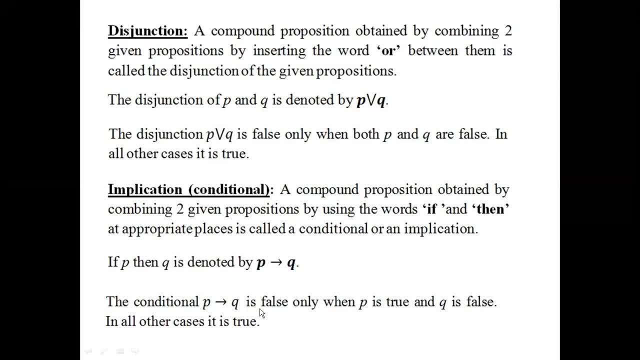 So we have P conditional Q, taking the truth value as false only when P is true and Q is false. This means P has the truth value 1 and Q has the truth value 0. So only when it is 1: 0 the. 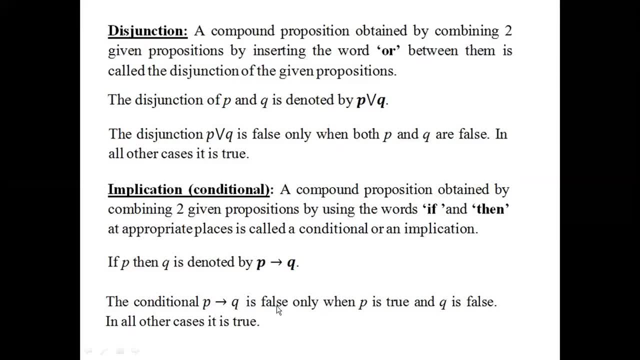 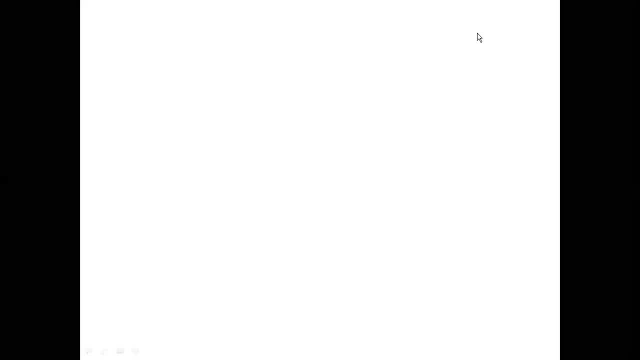 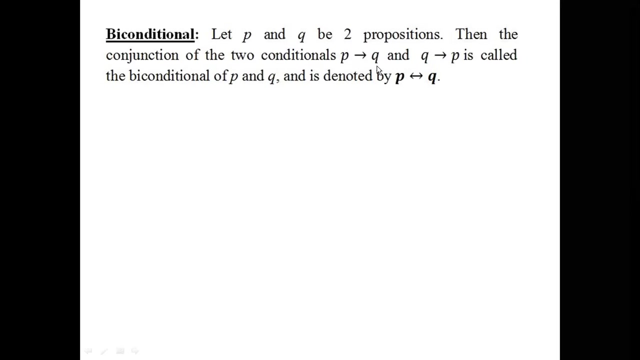 resultant P implication Q is 0.. In all other cases the truth value is 1.. Next definition is about biconditional. Let P and Q be two propositions. Then the conjunction of two conditionals- p conditional q and q conditional p- is called the biconditional of. 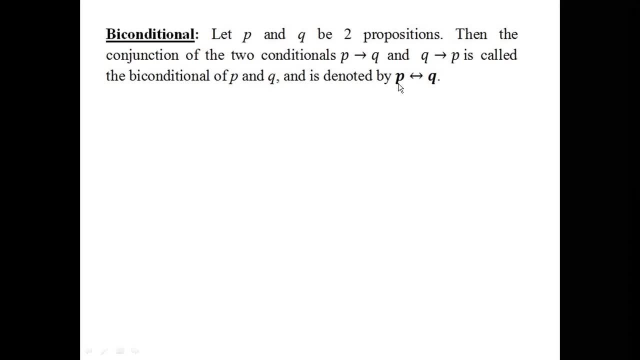 p and q and it is denoted by p arrow towards both the side q. We read this as p biconditional, q only. So we have two propositions given, which are p and q, then the conjunction of the two conditionals, that is, p implication q and q implication p. via conjunction We are doing. 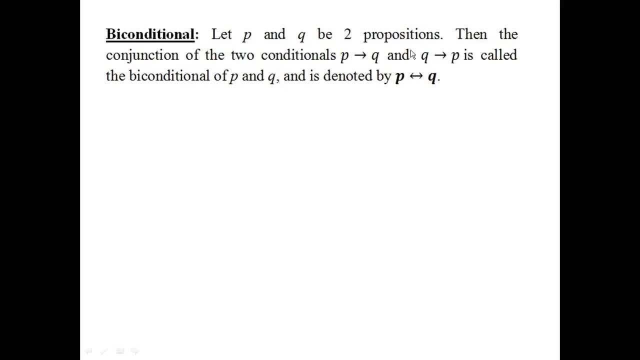 the conjunction means we are combining them by the notation and by the proposition and by the logical connective, and is called the biconditional of p and q, usually denoted by p. This is a symbol for biconditional q. It is read as: if p, then q and if 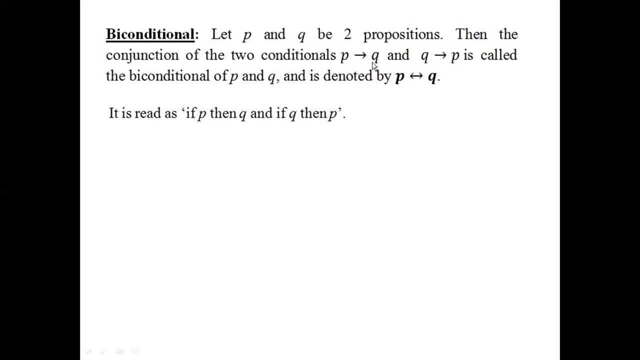 Q, then P. We have P conditional Q. No, it is read as if P, then Q and Q conditional P is read as if Q, then P. Next is about exclusive disjunction, The compound proposition notation in this form: P, we have a V and there is a underline below it, Q, read as either P or Q. 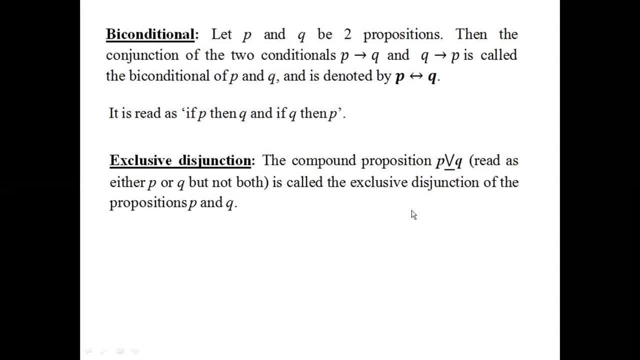 but not both is called the exclusive disjunction of the propositions P and Q. So this notation is usually read as exclusive disjunction of the two propositions P and Q, and usually read as either P or Q, but not both Equivalently. exclusive disjunction of P and Q is true only when either P is true or 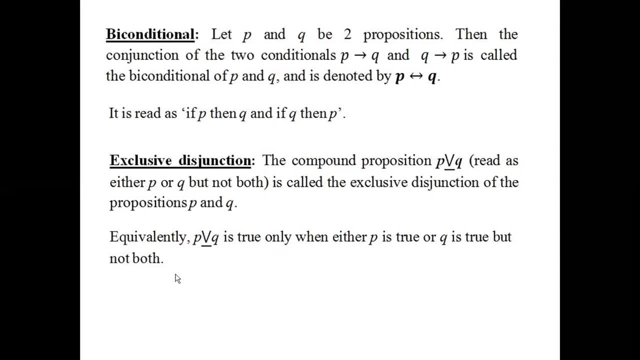 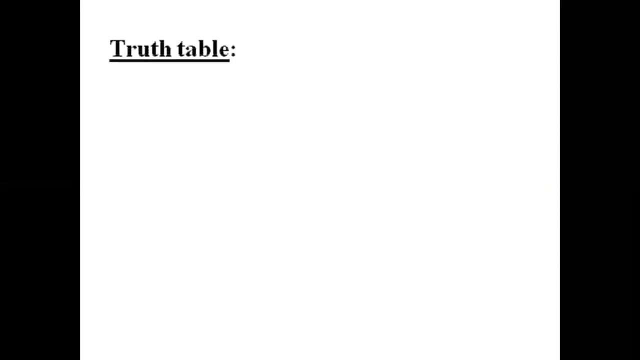 Q is true, but not both. So this is the symbol denoted for exclusive disjunction and this P exclusive disjunction. Q is true only when either P is true or Q is true, but not when both. Next we will see the truth table for all the notations that we learned. now The logical: 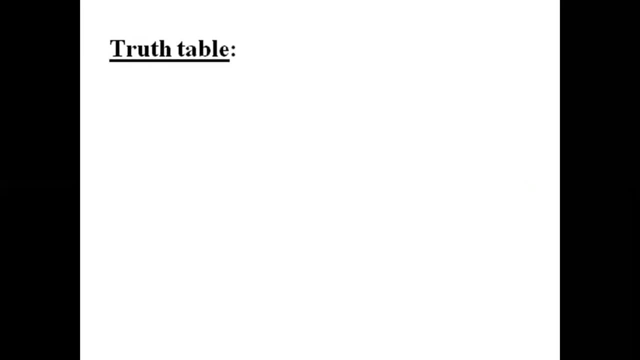 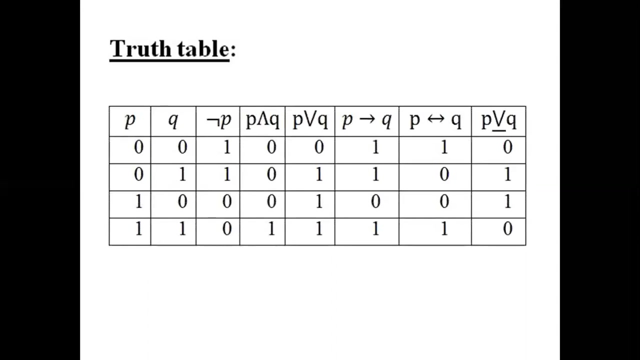 connectives. that is negation, and or if and only if. if, then So for all that, we'll put it in the form of a table and understand how the truth values are represented. So this is the table. for this, I have taken two propositions, P and Q. We fill the values. 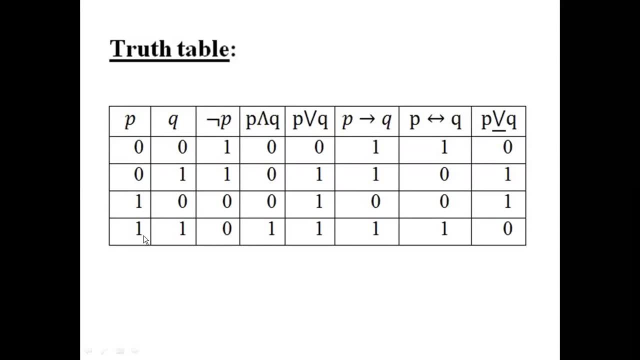 starting from 0 0 0, 1, 1 0, 1, 1.. That is, when both P and Q are false. P is false, Q is true, P is true, Q is false. and finally, when both P and Q are true. So negation P You have. 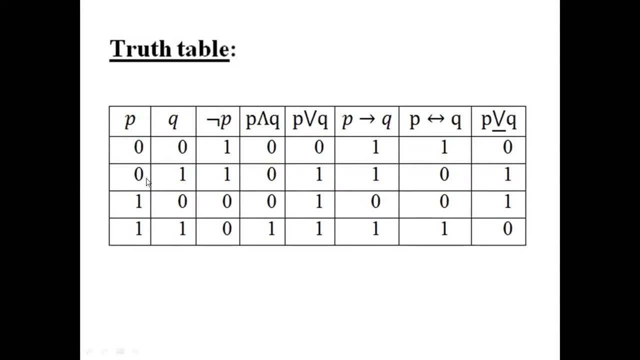 0.. So negation P gives you 1.. If you have 1, negation P gives us 0. Then the next one is P and Q. P and Q are the conjunction of P and Q. So conjunction of P and Q. 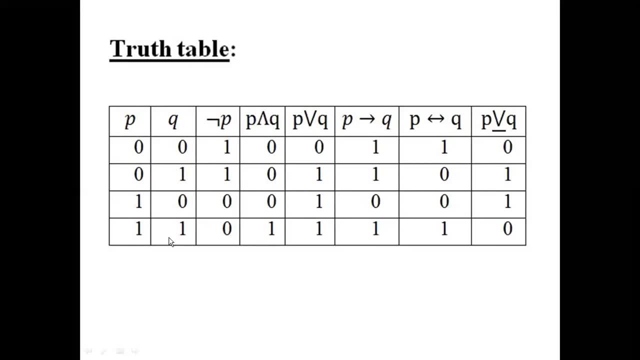 When is P and Q true? Only when both P and Q are true, Its truth value of P and Q is also 1.. Only when both P and Q has a truth value 1, the truth value of P and Q will also be 1.. 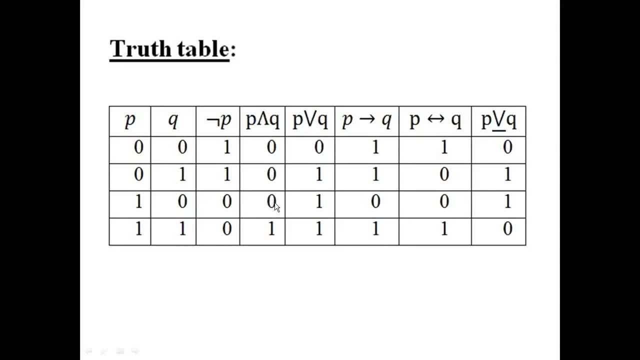 In all other cases, the truth value will be 0.. Similarly for P or Q: P or Q is false only when both P and Q are false. In all other cases, the truth value is 1.. That is it is true. 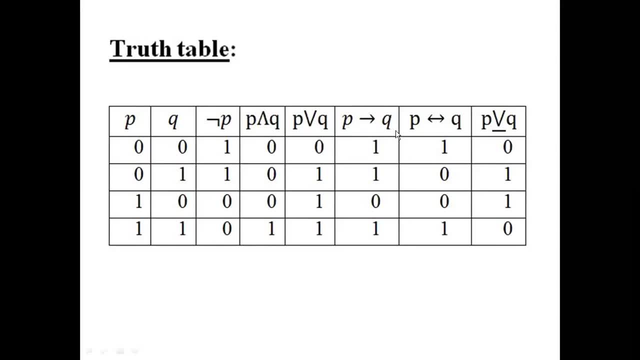 Then we have P. P implication Q, Recalling from the definition what we learnt for implication P. implication Q is false only when P is true and Q is false Only when P is true and Q is false. P implication Q is false. 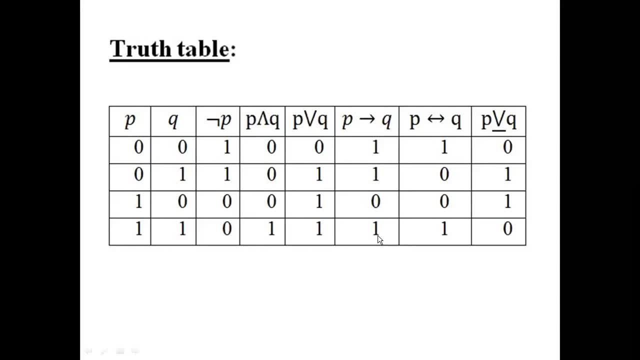 In all other cases it is true. Then P biconditional Q, Recalling from the definition, P biconditional Q is true when both P and Q are true or both P and Q are false. So both P and Q should be false or both P and Q should be true. 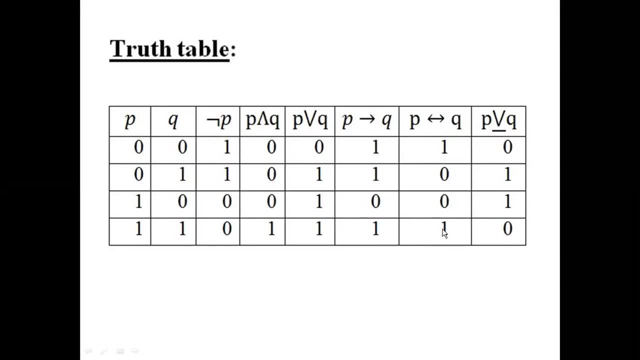 Then only P biconditional Q will be true. It is having the truth value as 1.. Only when both P and Q are 0s, Only when both P and Q are 1s. The rest of all cases it is 0.. 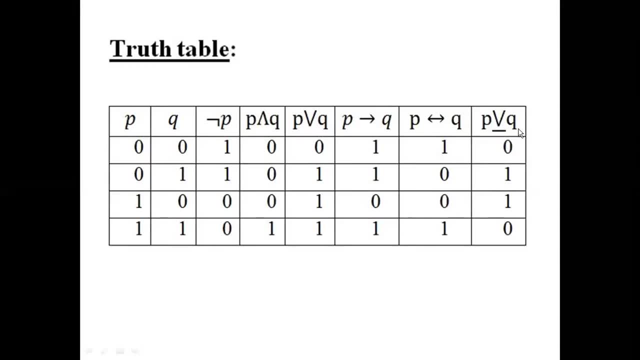 Then finally P, exclusive disjunction Q. It is usually read as either P or Q, but not both. So this is true when either P is true or Q is true. Either P or Q should be true only when its truth value is true or 1.. 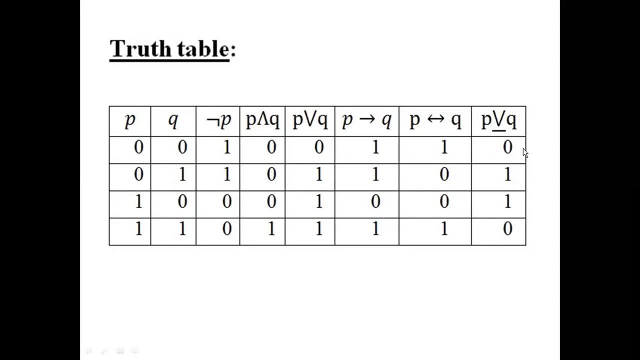 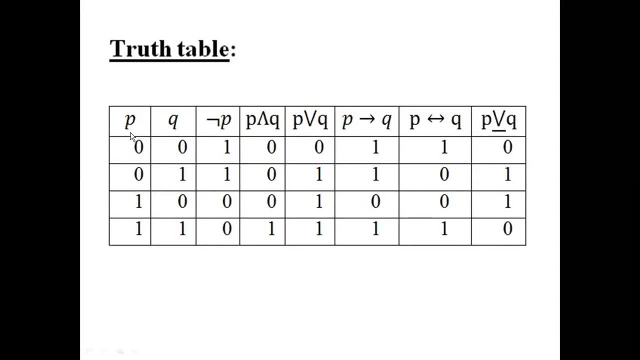 So this is how we write down the truth table. I have taken two propositions for that is P and Q here. So for P and Q we are doing this table. Similarly, if there is one more proposition or two more propositions also, we will be able to implement in the same manner and obtain the truth table. 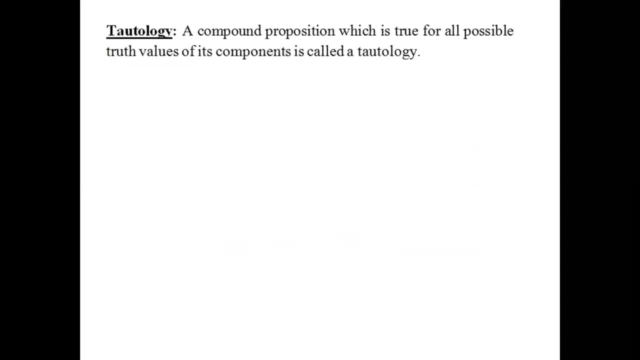 Next we will know about TAU-TAL. A compound proposition which is true for all possible truth values of its components is called a tautology. So we simplify the compound proposition and the simplified form of the composition proposition is the truth value one in all possible truth values of its components. then such a compound 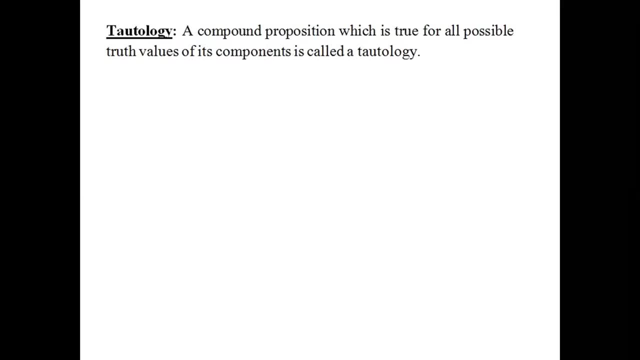 proposition is called tautology About contradiction. a compound proposition which is false for all possible truth values of its components is called a contradiction or an absurdity. So we say that if all the truth values of each components are zeros, then such a compound 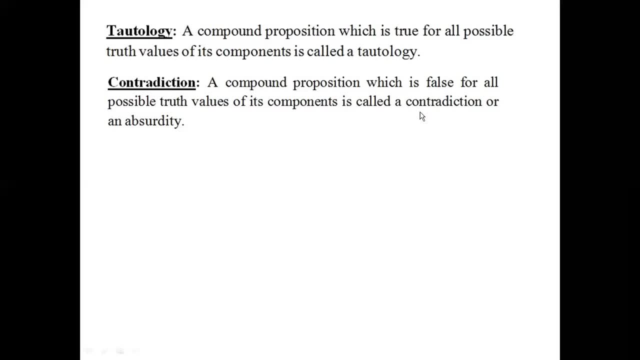 proposition is a called is called as contradiction contingency. a compound proposition that can be true or false depending upon the truth values of its components is called a contingency. So the table will have a mixture of truth values, one and zeros. so it can be either: 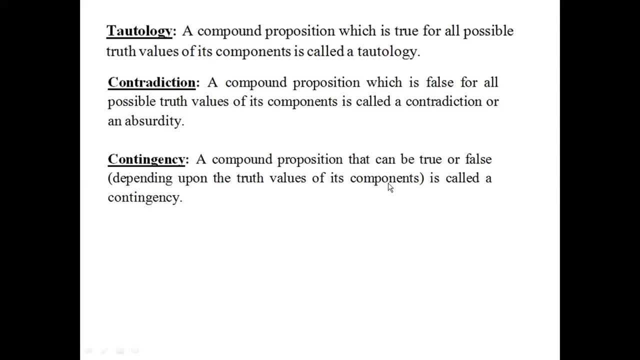 true or false, depending upon the truth values of the components. Then such a compound proposition is called contingency. Next we have logical equivalence. Two propositions, u and v, are said to be logically equivalent whenever u and v have the same truth value. or equivalently, we can write down the bi-conditional, the bi-conditional u. 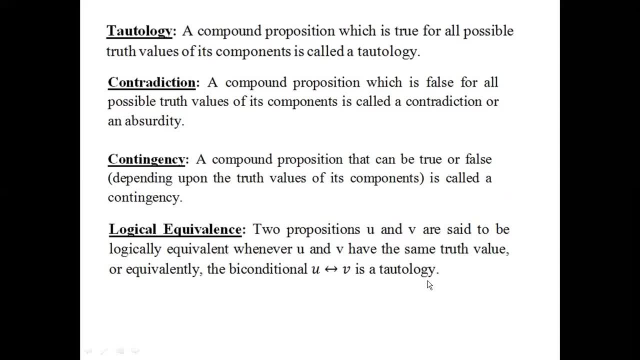 bi-conditional v. So for the given proposition, when you perform u bi-conditional v, if the truth value of each components are one, then we say it is a tautology. So if the bi-conditional is a tautology, we can conclude that u is logically equivalent. 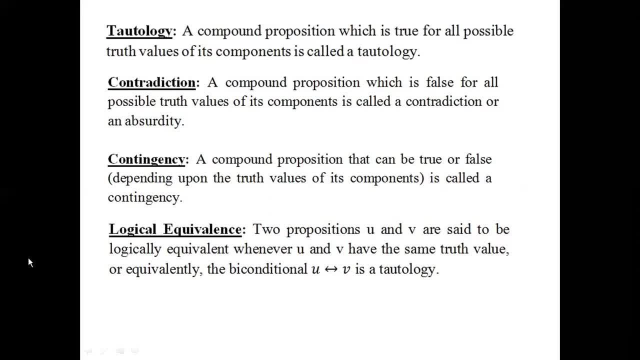 to v Or another way. if we have to prove the logical equivalence of two propositions, u and v, they are said to be logical. So we can conclude that u and v are said to be logically equivalent if they have the same truth value. 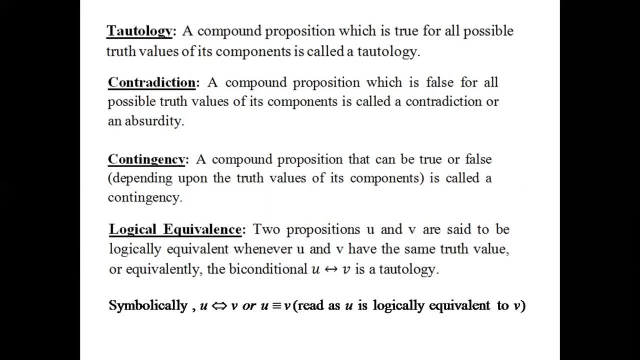 Symbolically it can be written as: u is logically equivalent to v or u is logically equivalent to v. So these are the symbols that are used here. implies and implies by symbol or the three parallel lines. So these two are the notations for logical equivalence. 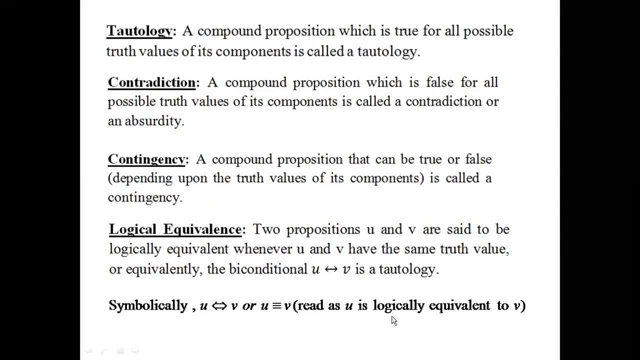 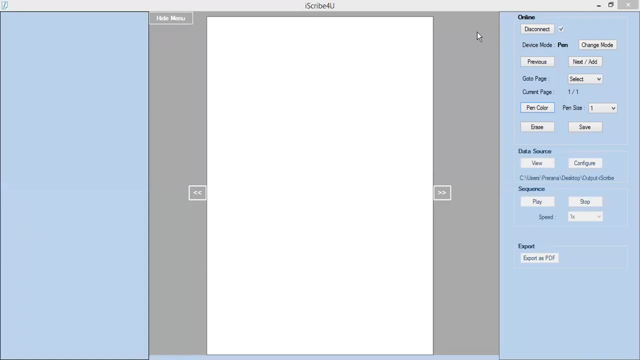 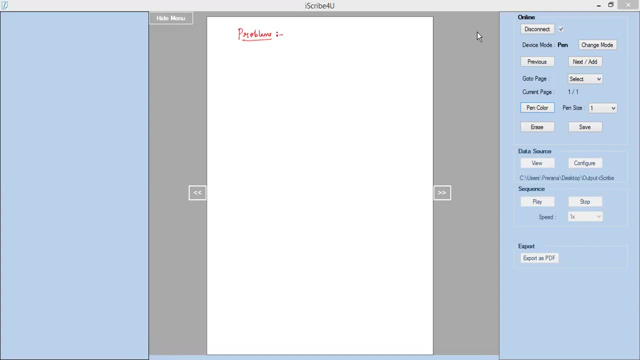 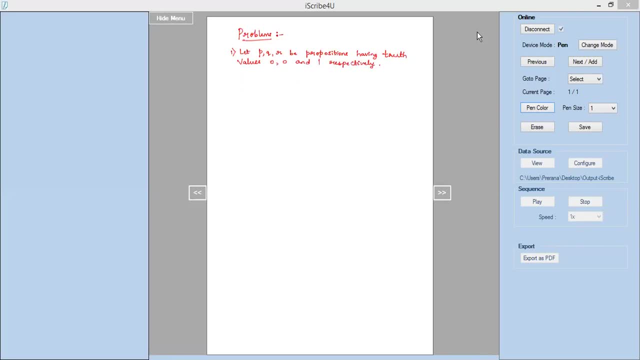 Having truth values 0,, 0 and 1 respectively. Find the truth values of the following compound proposition: Find the truth values of the following compound propositions: Find the truth value of the following compound propositions: Find the truth values of the following compound propositions: 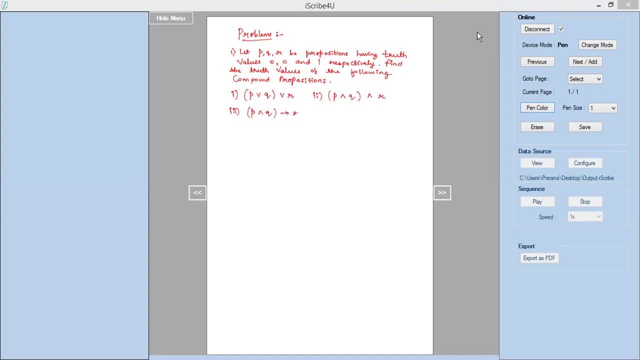 Find the truth values of the following compound propositions. So, given the truth values of P, Q, R as respectively 0,, 0 and 1,, we have to find the truth values of the given compound propositions. So we'll just do one by one. 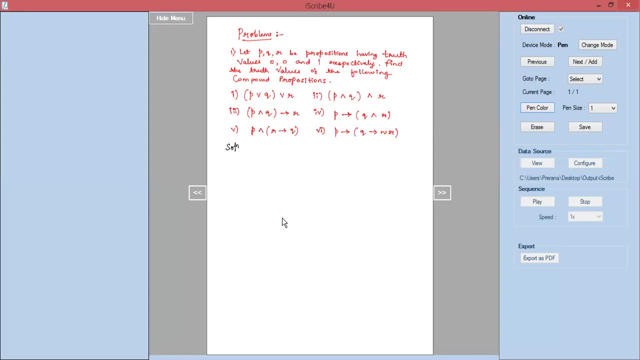 We'll frame a small table in each of the cases and do P Q R. P Q R has the truth values 0, 0 and 1.. 0, 0, 1.. The first one we have to find is P or Q. 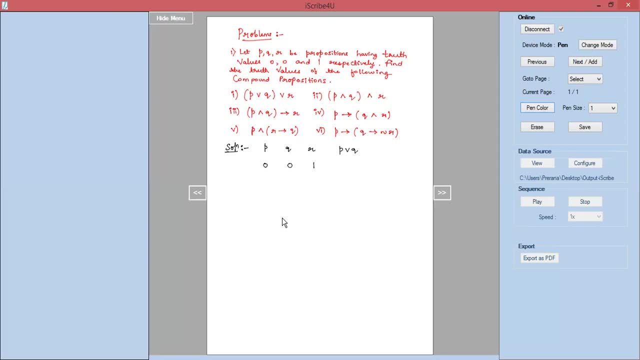 So first we will be finding P or Q, and then we will use P or Q or R, P or Q or R, So we'll just frame the table and do it so that things will be easy for us to understand. And then, so p q, r are given respectively as 0, 0, 1. we have to use p or q. recall the definition for. 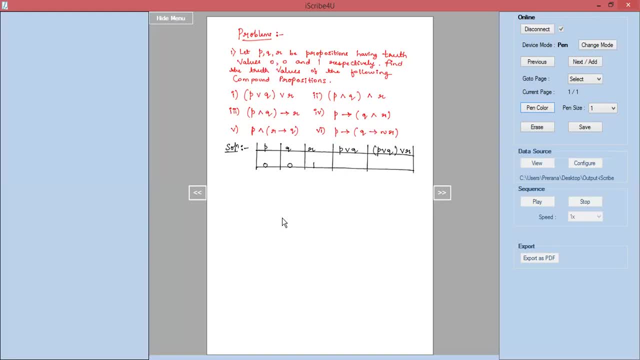 disjunction p or q, p or q. both p and q have the truth value 0 and 0, so p or q will also have the truth value 0. then we have p or q or r, so p or q has the truth value 0, r has the truth value 1. 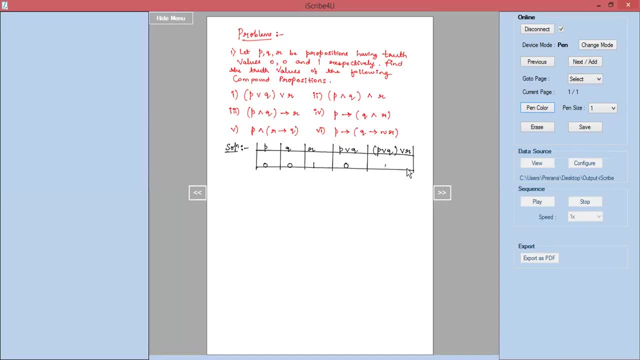 so 0 or 1 gives us 1 gives us 1. so this was the first sub question for this. similarly, we have to do the remaining second one, second, one, second one. we have to do p and q and r. first we will do p and q, then we will implement p and q. 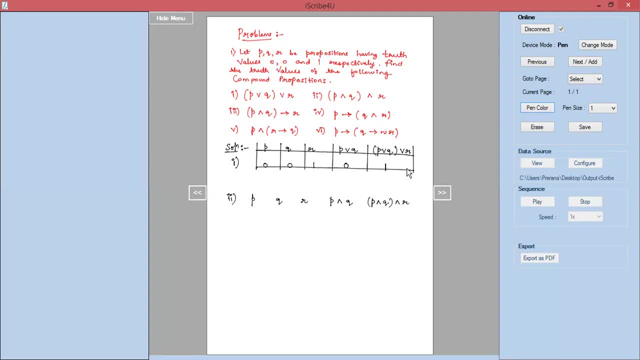 and r, p and q and r. so truth value of p is given as 0, truth value of q is given as 0, r truth value is 1, and for p and q. p and q, both are zeros, so resultant for, and that is constant- conjunction is also 0. you have to remember the rules for each one of them for conjunction. 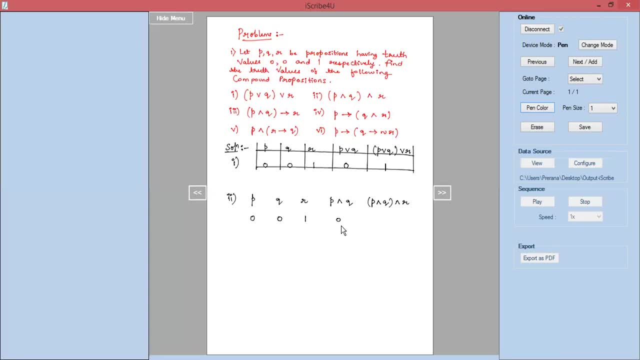 disjunction implication and all that. we have to remember the rule. so rule for p and q is when both p and q are 1, only then p and q is also 1. the rest all cases it is 0. that is why we have 0 here now: p and q and r, p and q and r. 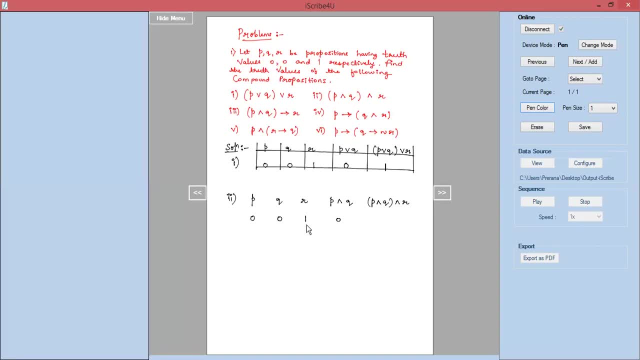 is also 0, because 0 and 1 we are doing only when both are 1. the resultant would have been 1, so this is 0. we have the resultant as 0 in the conjunction. in the conjunction then we have third one. i will write down the truth values of p, q, r. that is 0, 0, 1 as it. 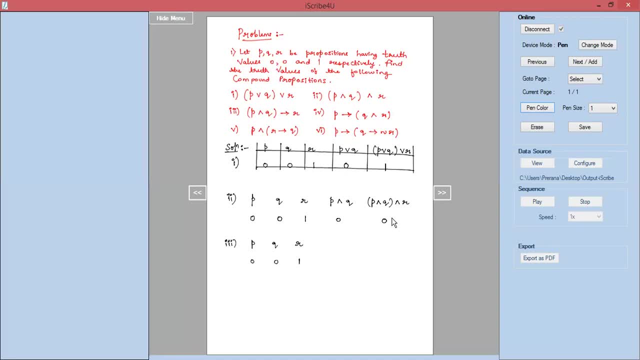 is. Then we have to find P and Q conditional R. So first we will do P and Q, which is 0, because we have already seen it in the previous case also, P and Q is 0. We have to now imply P and Q conditional R. we have to do: 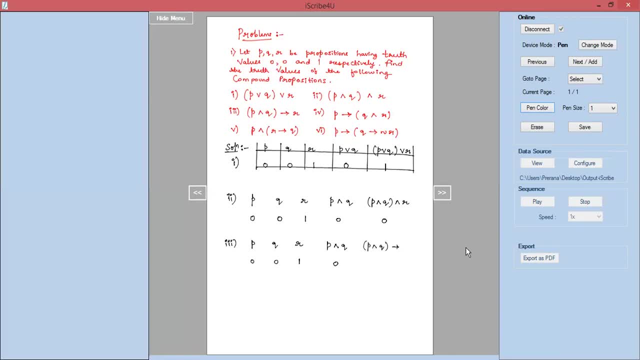 So P and Q, conditional R. Conditional R we have to implement: P and Q is 0.. 0. conditional 1. 0. conditional 1 is 1. 0. conditional 1 is 1.. Remember the implication Only when P is true and Q is false. 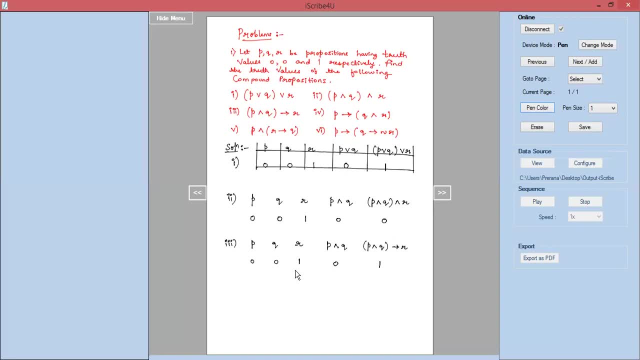 The resultant P conditional Q is false. Rest all are 0s. So only when you have 1, 0 the resultant is 0. Rest all cases are 1.. That is the definition of a conditional. That's the reason we have 0, 1 here. 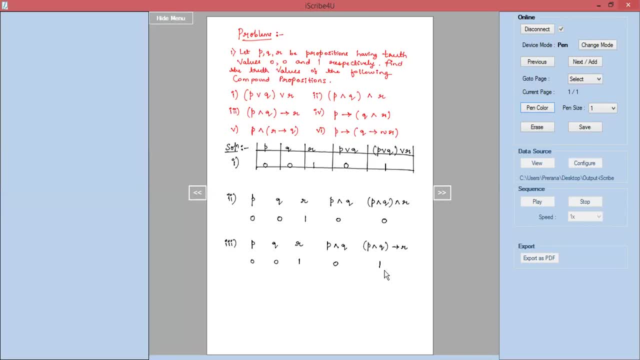 P and Q is 0.. 0, conditional 1 we are doing, The resultant is 1.. If you have 1, 0, then only resultant is 0.. Now, moving ahead to the fourth one. Fourth one: we have to perform P, conditional Q and R. 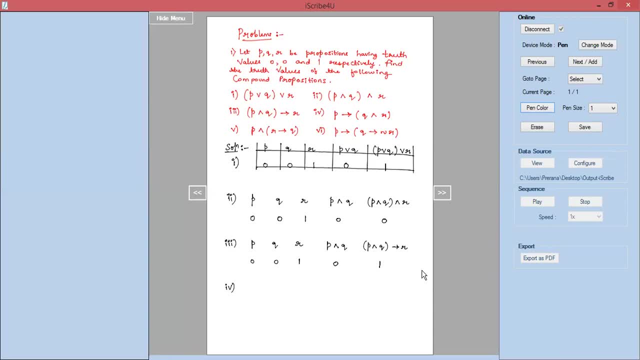 So first we have to do Q and R? no, First we have to do Q and R. Firstly, we will write on P Q R and its truth value. Truth values are 0, 0, 1 respectively. First we need to perform Q and R. 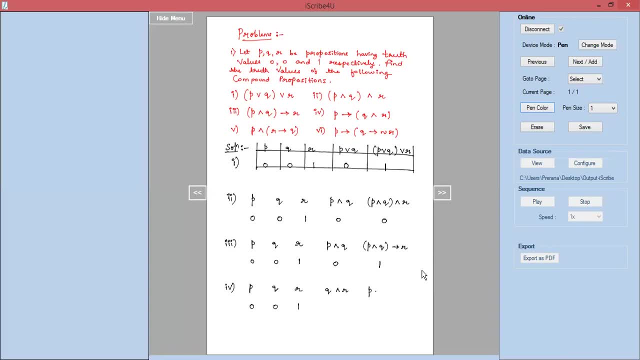 Q and R, Then we will have to do P, conditional Q and R. What is Q and R? Q and R And means conjunction. Conjunction is 1 only when both Q and R are 1.. One of them is 0, so resultant here is 0.. 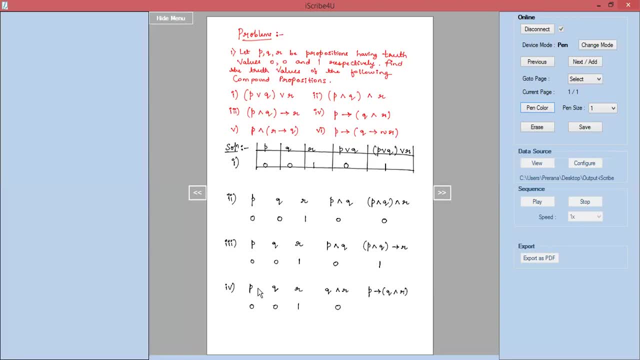 P conditional Q and R. P is 0.. Q and R is 0.. So 0 conditional 0 is 1.. If you have P as 1, Q and R as 0, then it will be 1, 0. 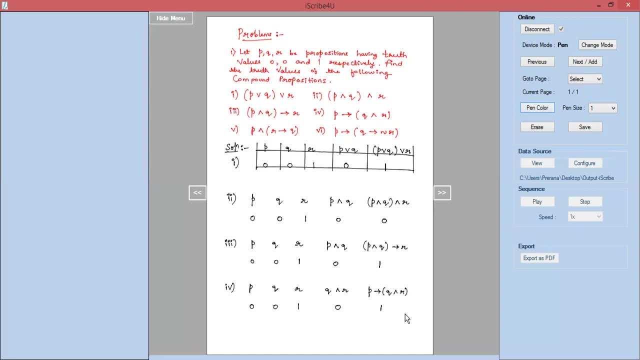 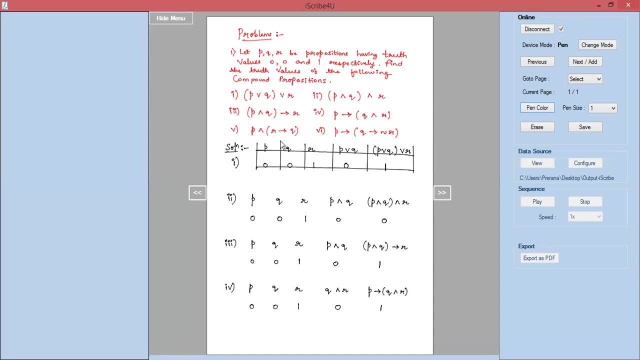 Fifth one. Fifth one: we have to do P and R conditional Q, R conditional Q. First, we will have to perform R conditional Q, followed by we have to do and with P. I will just do that in the next page, Due to the fact that we went through them. 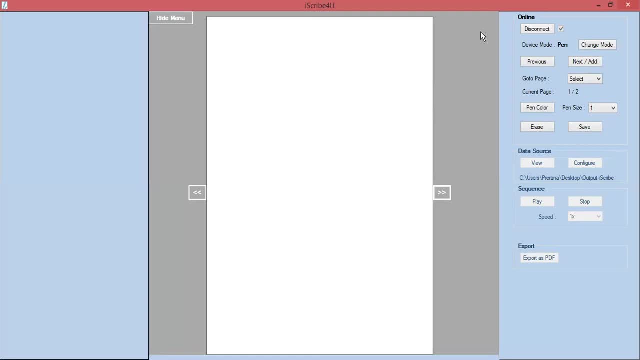 So, in a general zoo and sort of亲等 covid-19 situation, We are expected- This is a lie, I'm expecting- to get negative grades and positive�יs a you Out of all of the we see for ourselves. So what is therefore? 1 for you. 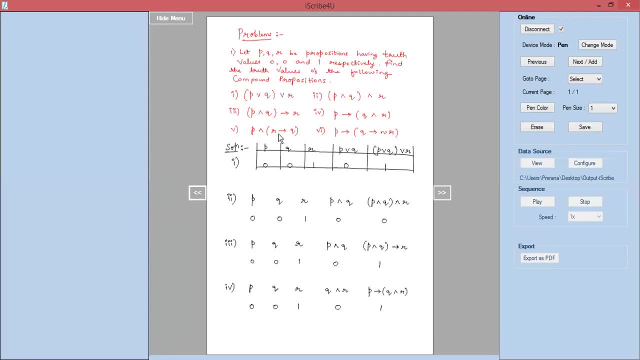 Correct. Why so mostly positive and always not positive? That is of course a part of the solution. It is decided There are all possibleım out there as rough. so 5801, what we have to do R, then I have to do R, conditional Q and then AND with P Right now. So first we will write. 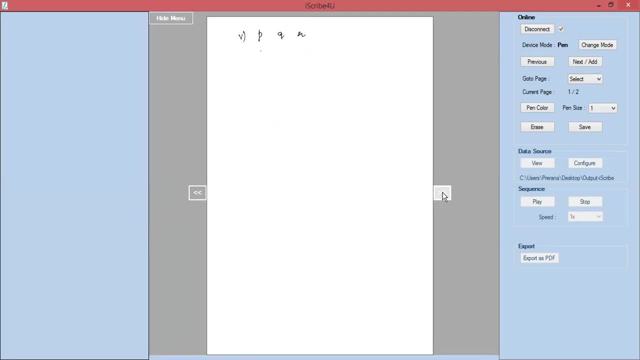 down: P Q R has the truth value 0, 0, 1.. Then we have to perform R conditional Q, followed by P and R conditional Q, P and R conditional Q. So R conditional Q gives us 1: 0.. Read it reversely: 1: 0, because we are doing R conditional Q, So 1: 0 is 0 in the conditional 1: 0 is. 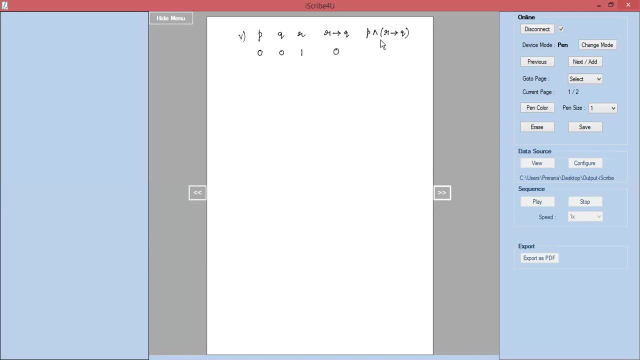 0 in the conditional. Now we have to perform P and R conditional Q. P is 0. R conditional Q is 0. And between them both are 0s, means resultant is 0 in the conjunction. Now the next one, That is sixth one: P conditional. 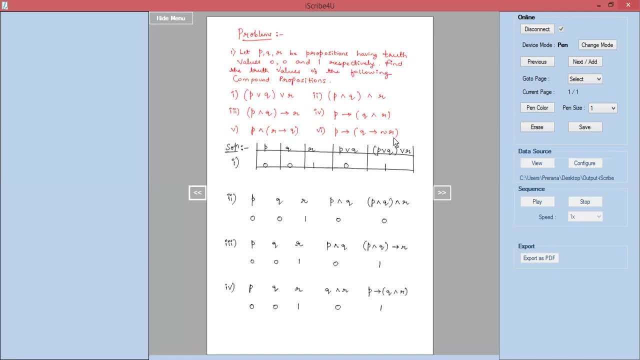 Q- conditional Negation R. So after we have written R, we have to first write down negation R, Then we need to perform Q- conditional negation R. Then we have to imply P- conditional, Q- conditional negation R. Do it according to the brackets. We will do one by one. So firstly we have 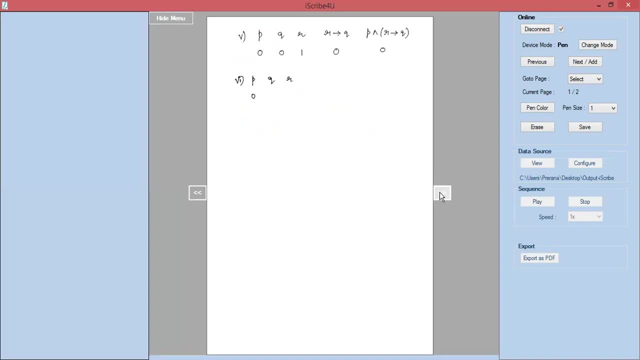 to write down the truth values of P, Q, R, which are 0, 0, 1 respectively, And then we have to first do negation R, Then we have to implement Q conditional negation R, Then finally, P conditional, Q conditional negation R. Right, So negation R will be 0.. If you have the truth value as 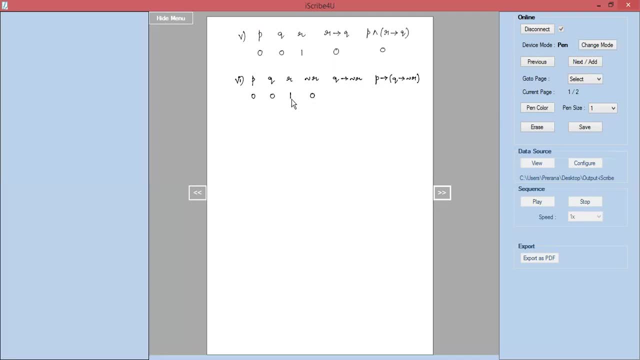 1, negation of that value will be 0.. If you have the truth value of R is 0, then negation R will be 1.. Why is that versa? So R has the truth value 1.. That's why negation R has the truth value 0.. 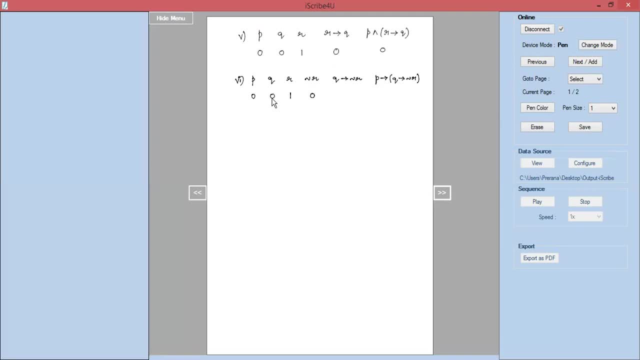 Next: Q conditional negation R. Q is 0, negation R is 0.. Q conditional negation R will be 1.. In conditional only when you have 1: 0, resultant is 0. Rest all cases it is 1 only So that. 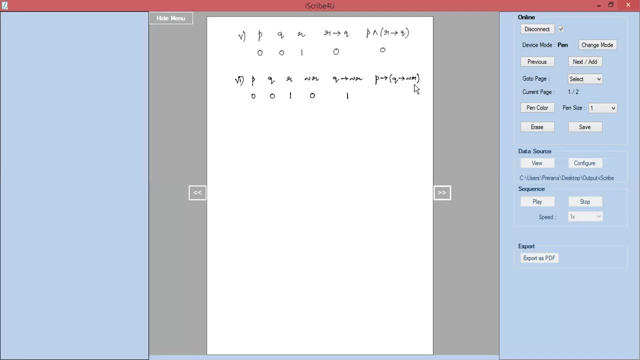 is why Q conditional negation R is 1.. we have P conditional of Q conditional of negation R, So P is 0, Q conditional negation R is 1.. So 0, 1 gives us 1.. 0, 1 gives us 1.. So this was the basic problem which I took. 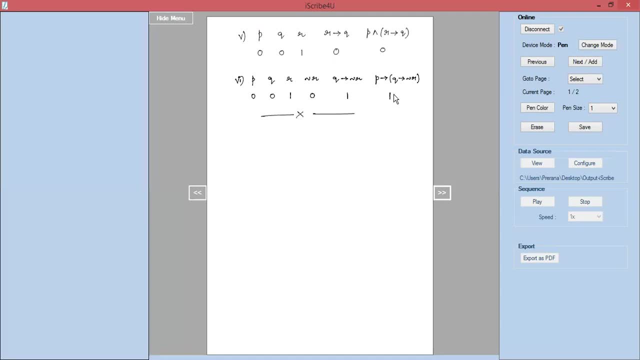 to make you understand about the simple definitions of conjunction, disjunction, negation, implication and all Second problem. show that, show that for any two propositions, for any two propositions, P and Q, P and Q, first one, P exclusive, exclusive or Q. P exclusive or Q or P biconditional. 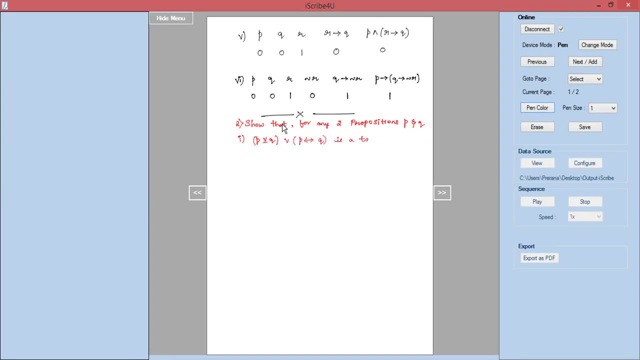 Q. is it ontology? Second, Second: one P exclusive or Q and P conditional. Q is it contingency? Third, one P exclusive or Q and P biconditional Q? Q is a contradiction Is a contradiction. So again, using the truth table, we will be. 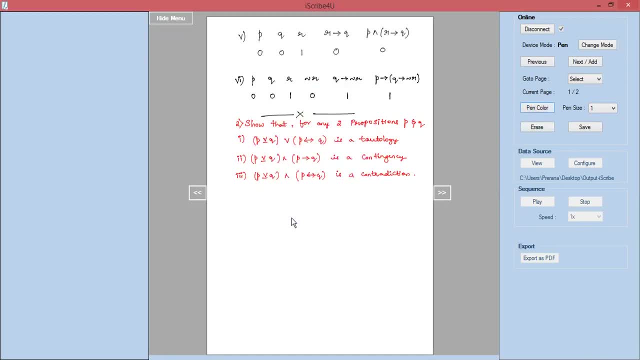 able to do the problem. So let us see how to do Solution. Solution will form a truth table Right now. starting from PQ, you observe that only P and Q are equal. So P and Q are the two propositions you are having. So we will in the table with only P and Q. PQ will. 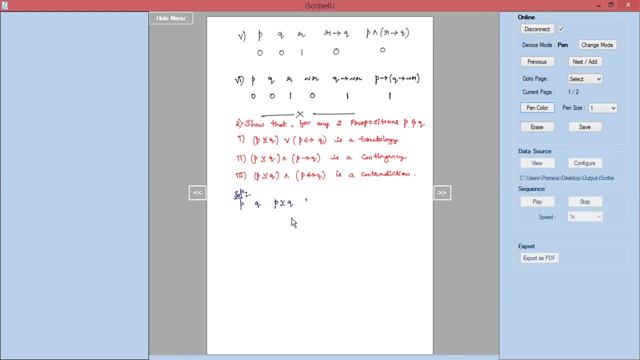 be need of P exclusive or Q, will be need of P biconditional Q, P biconditional Q And in the third one, if you observe, we also have P exclusive or Q will be need of P exclusive or Q. We also have in the second one, P conditional Q. So let us frame these and do the first. 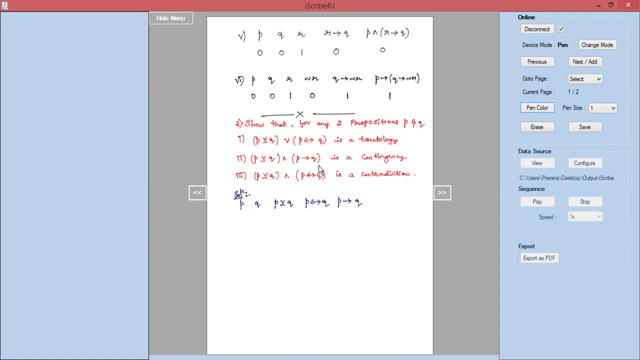 second and the third part of the problem. We will write out the truth values of all these, first, starting from 00, 01, 10, 11.. These are the different possibilities of the truth values that exist for two propositions. This is the truth value of the truth values. So 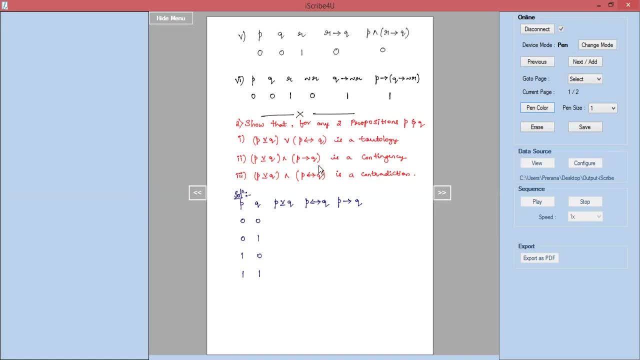 why it is called truth value, Because this is a fact and this has come out of the problem. positions P and Q. Now what is the definition of exclusive, or P? exclusive or Q? we have to find out. P exclusive or says the rule that it is true only when either P is true? 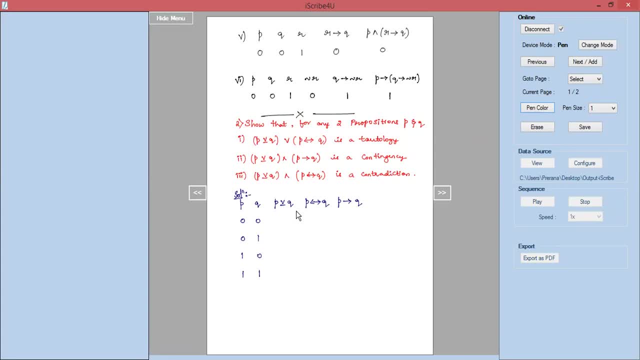 or Q is true, but not both. So either P should be true or Q should be true. Then only P exclusive, exclusive or Q is true. This is P exclusive or Q is true only when either P is true or Q is true. So here are the true values for us, Rest all cases it is false. P biconditional. 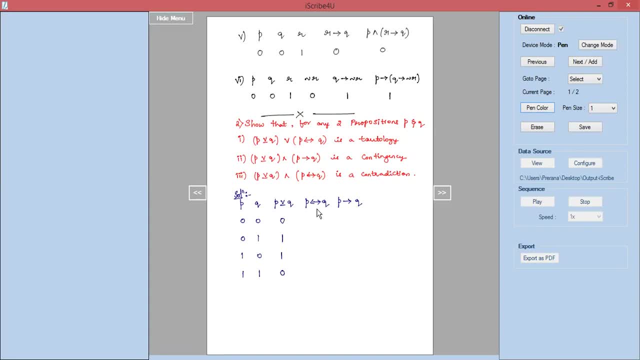 Q. We have P biconditional Q rule, as P biconditional Q is true only if both P and Q are true or true. Now, both P and Q are false. Both P and Q should be true or both P and Q should be false. So 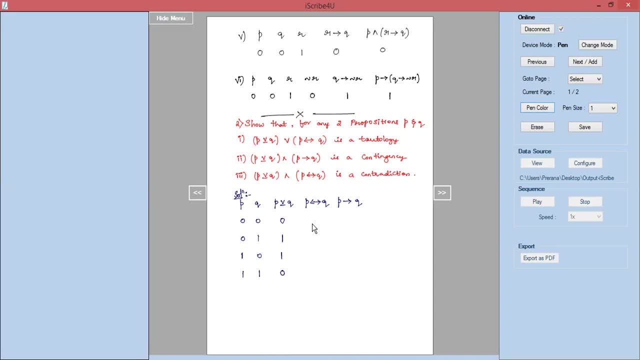 it is in the first case you observe both P and Q are false. So P biconditional Q is true. P and Q are both true in the last case, So P biconditional Q is also true. Rest all cases: it is false. Rest all cases: it is false. 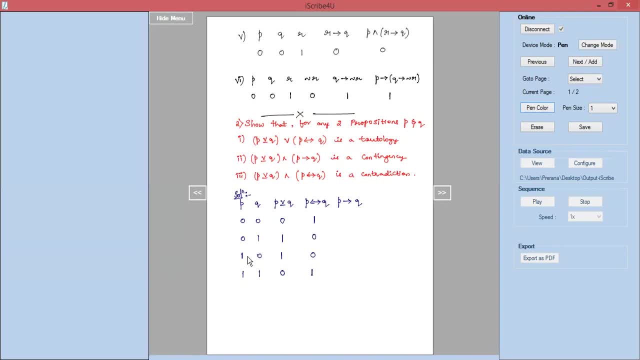 Then we have P conditional Q. P conditional Q only when 1, 0 we have, The resultant is 0. Rest all cases, it is 1.. So only when it is 1, 0 it is 0. Rest all cases, it is 1.. 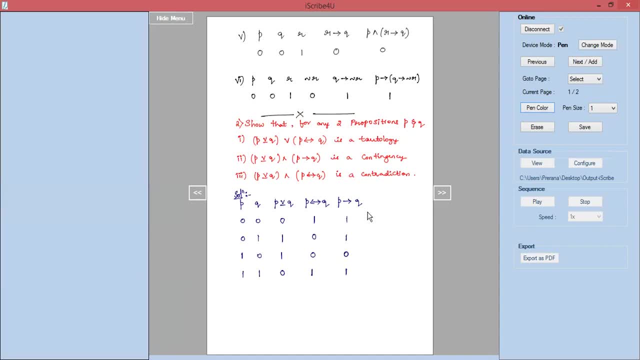 So this is for P conditional. Now we will have to do one by one. First case: is P exclusive or Q, or P biconditional, conditional Q? So we will call these expressions P exclusive or Q as X or convenient. Similarly we will call P biconditional, Q as Y or convenient. So first one: are we performing X or Y? We? 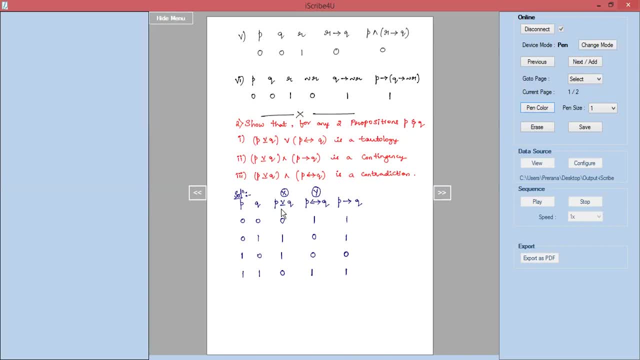 are performing X or Y. No, X is nothing but P exclusive or Q. Y is nothing but P biconditional, Q. There is OR in the middle, So we are performing X or Y. We are performing X or Y, So what? 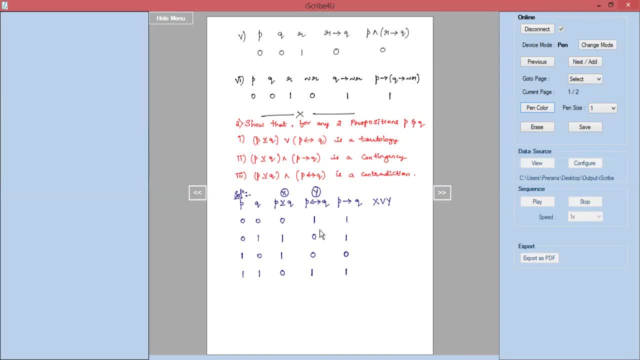 does X or Y give OR. That is disjunction. Disjunction says that only when both the truth values are zero, resultant is zero. If one of them is one, then the resultant will be one. So X or Y gives us one in all. 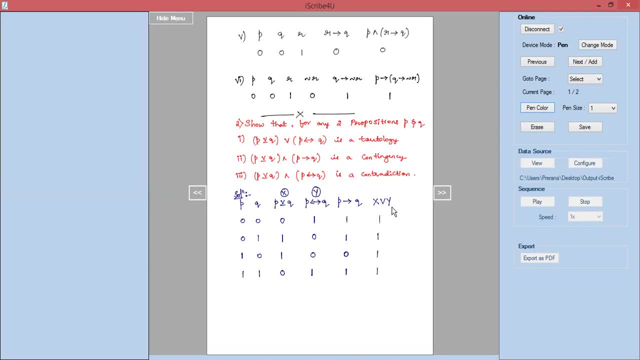 the cases here. X or Y gives us one in all the cases. Why it is because we are performing zero. one is one zero or one is one. one or zero is also one. one or zero is one, zero or one is also one. That is the definition for OR Disjunction. 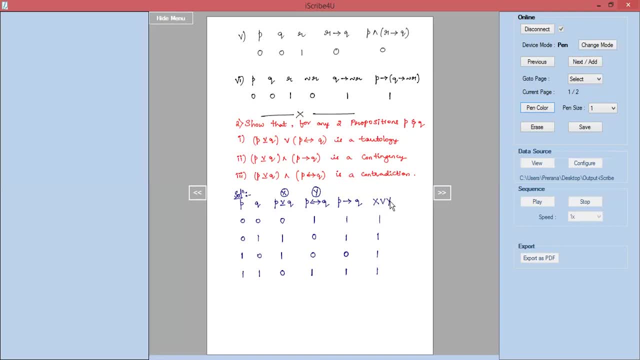 This is the answer for the first case. For the first case, this is the answer. Now for the second one: P exclusive or Q and P conditional Q. Here you have P conditional Q, no. So just for convenient, we will write down P conditional Q as Z. Just for convenient, we will represent. 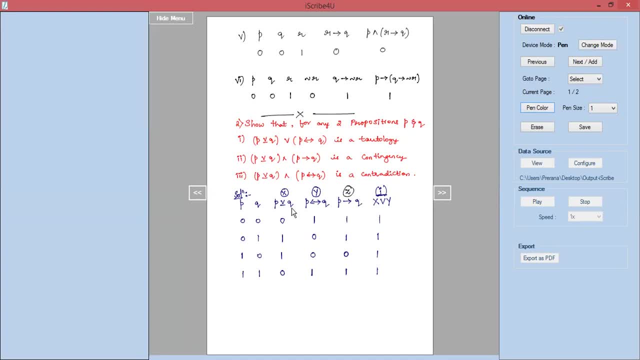 this as Z. So what are we supposed to perform? We are supposed to perform P, exclusive, or Q. That is X and Z. So we are supposed to perform X and Z. So we will do that: X and Z. We are working. So what does AND gives AND says that only when both the truth values are one. 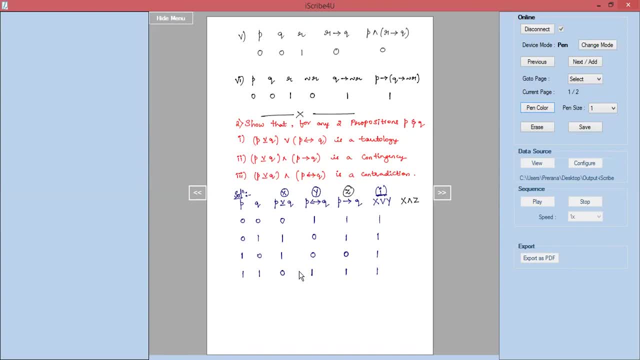 resultant is one. Rest all cases it is zero. So you have to look into this column. And then you have P, exclusive, or Q, That is X and Z, So you have zero, one, So resultant is zero. And the AND You have one, one, So resultant is one. And you have one, zero, So resultant. 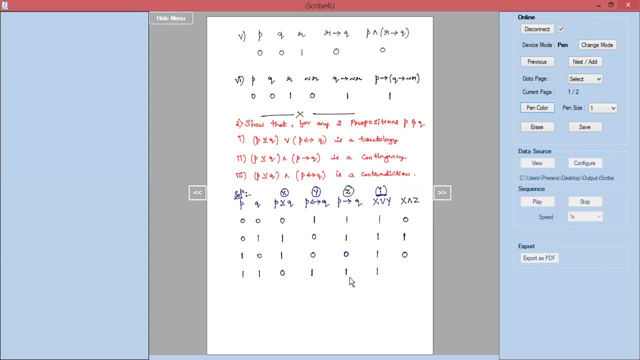 is zero, The last one is also zero and one Zero and one, also resultant, is zero. So, did you observe, it is a mixture of zeros and ones. This is the answer for the second case. We observe that it is a mixture of zeros and. 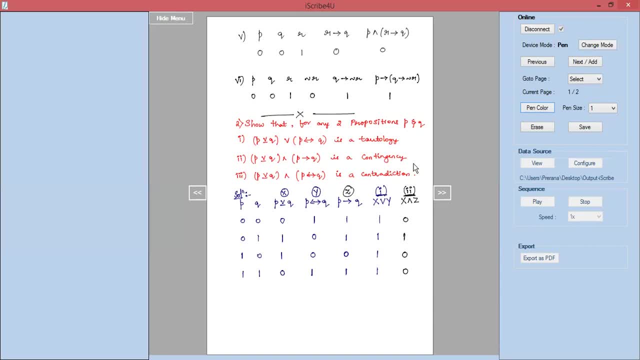 ones, which is nothing but contingency. Did you observe the answer to the first one, that it is all truth? values are all one, So first one is a tautology. Second one is a mixture of zeros and ones, So it is a contingency. Third one: I will leave it to the students. 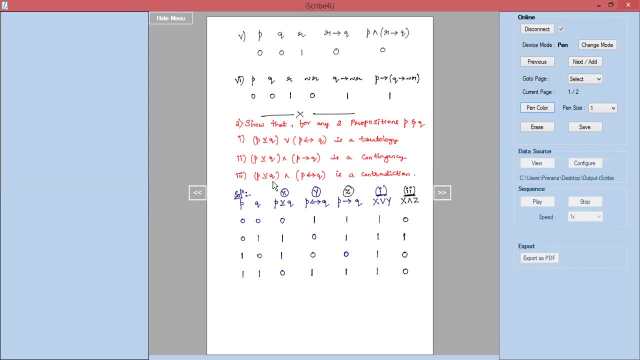 to do? We have to perform P- exclusive or Q, So resultant is zero. So resultant is zero, So resultant is Y, So resultant is 0.. We have to perform T- exclusive Q And T- bi conditional Q and show that it is a contradiction. Contradiction means all your. 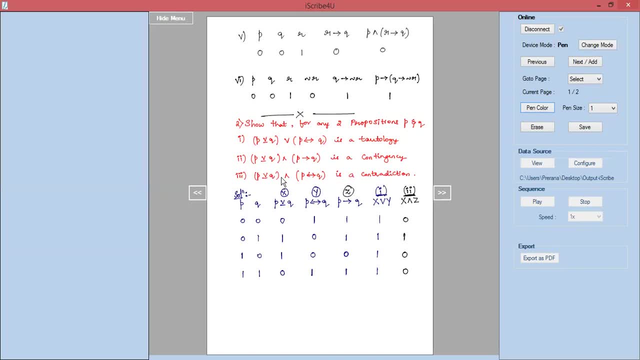 truth values should be 0. All your truth values. when you perform this compound proposition, The truth values in all the cases should be 0. So try doing that. I will conclude for first and second one. OK, first and the second results are: 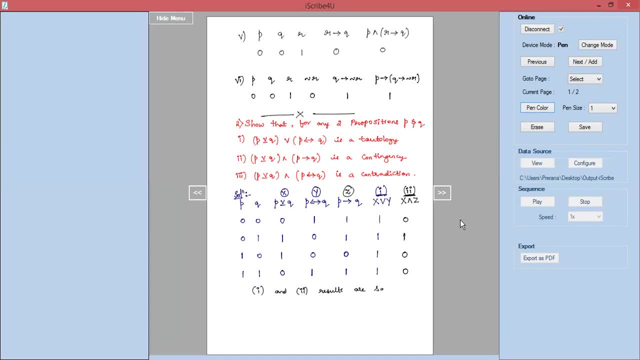 Why first and second results are satisfied. First one: we have proved the truth. values of all of them are 1.. So it is a tautology. Second one we have proved it is a mixture of 0s and 1s, So that is why it is a contingency. Third one: you have to do it by yourself. 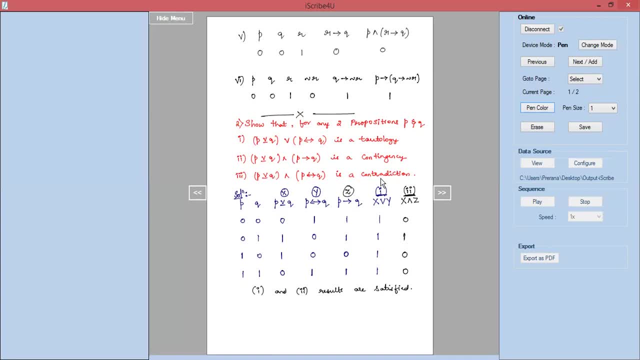 You have to prove and get the resultant as 0s in the proof table. when you perform this x and y, When you perform this x and y, your resultant has to be all 0s. So you can conclude it is a contradiction. We will do. third problem: Proving the resultant for a tautology. So 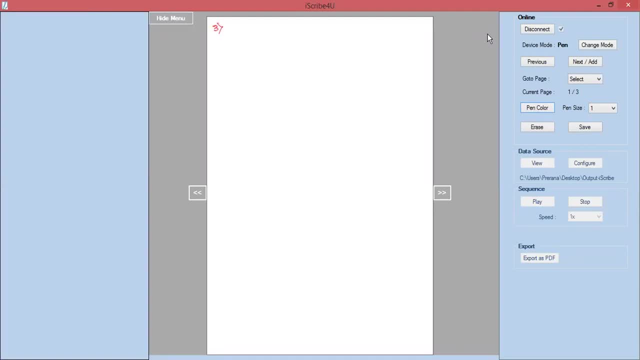 it is a tautology. Third one: prove that for any propositions P Q R, for any propositions P Q R, the compound proposition given by given by P or Q and P conditional R and Q conditional R, Put a big bracket for. 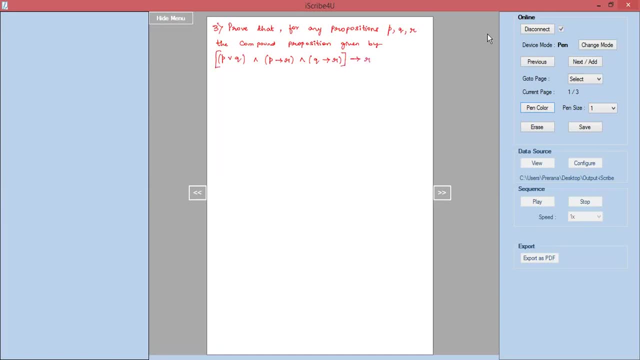 this Conditional R is a tautology- Is a tautology, So we have to prove the condition. We have 3 compound propositions- P, Q, R- for us, So we need to perform the compound proposition P or Q and P conditional, R and Q conditional. 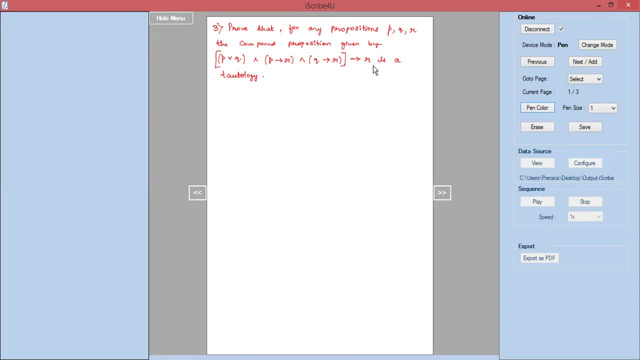 R, The whole thing. conditional R is a tautology. we have to prove Tautology is a conditional R. Tautology means the resultant proposition should be all 1s, Having the two values as all being 1s. So let us start performing this using the taut table. Solution: P, Q, R, P. 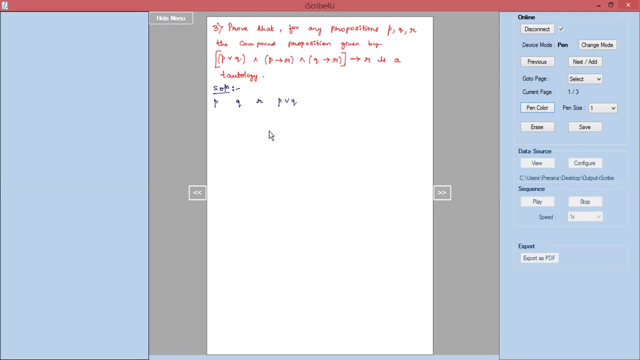 or Q underneath P or Q. then we want P conditional R. Then we have to perform Q conditional R. Then we observe that we have P or Q and P conditional R and Q conditional R. So just put a right 3 Feet with all those arrows. So pick that value and then pensa that you are interested. 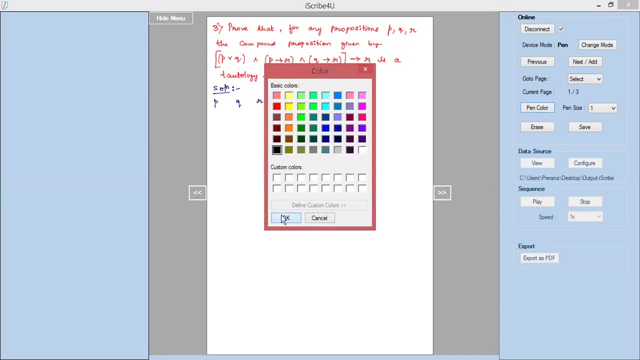 in düring the right area ahead. And third, the decision is your choice from here, So we. So, just for simplification, I can assume these as x, y and z. Just to be on the simpler side, I'm assuming this proposition as x, y, z respectively. 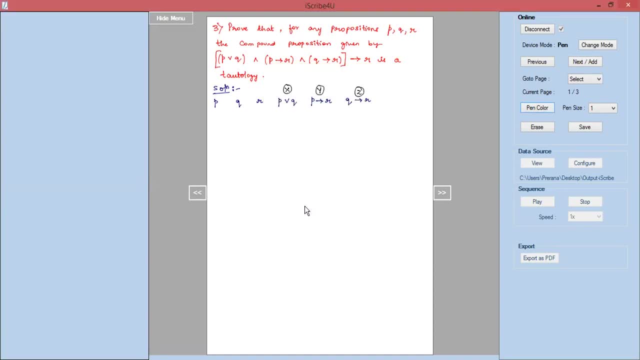 So that you have to now perform x and y and z. No x and y and z. Still the work is not over. So this big bracket becomes x and y and z conditional, or you have to back. Okay, we'll just do that. 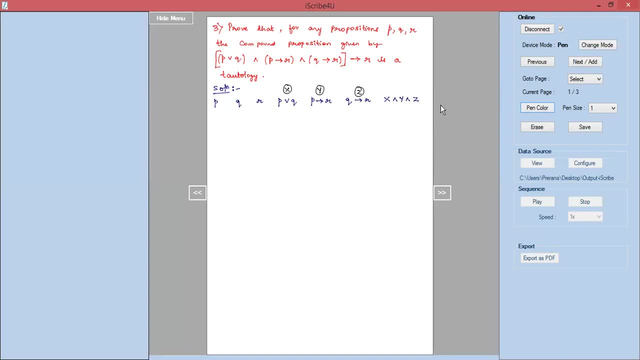 If possible, try to do it in one particular columns, one set of columns, so that it is all in one line. Okay, so we have the right on the truth values of each one of these first. Hey, let's put the right value in a documentation. 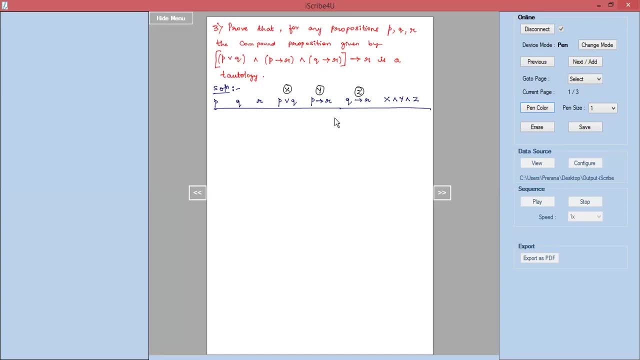 Hmm, Both of them are areas where you can see clearly And, Are you happy? practice on your topic? Okay, great. Well, it's going to do the job myself, Is everybody Okay? So fast forward. Mmm, Okay. 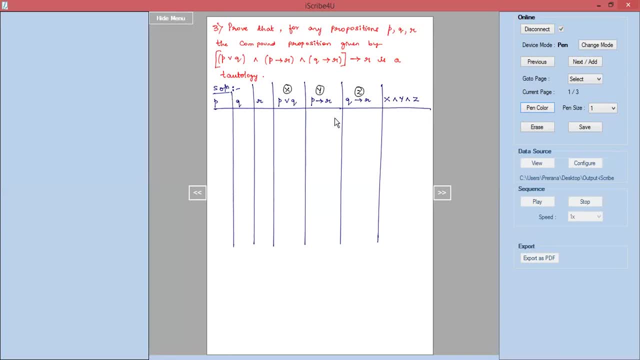 we will write down the truth values now: p, q, r. so 0 0 0 0, 0, 1 0, 1 0, 0, 1, 1. then we have 1 0 0, 1 0, 1 1, 1, 1, 0 and finally 1 1 1. so eight different possibilities are there. 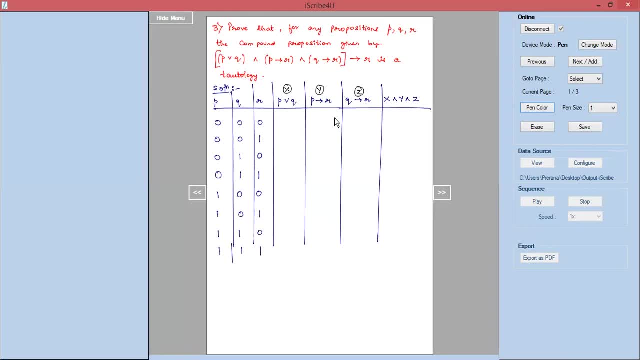 so these are the eight different possibilities. try to go in an order so that you will not mess up and do wrong. okay, only when you go in an order, things will be always easy for us to proceed. so we have to now perform p or q. you have to now perform p or q, or so any one of them is one. 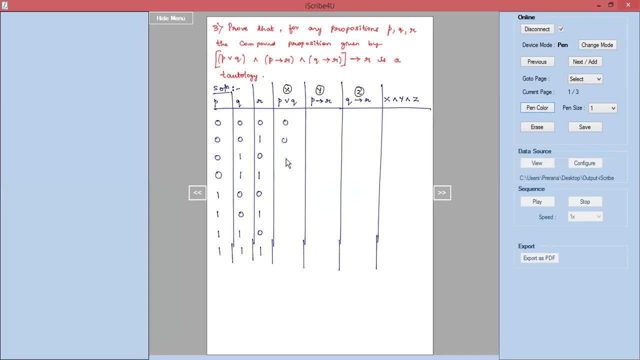 resultant is one, so we have 0, 0, 1, 1, 1, 1 1. or says that when you are looking for p and q, look into the first two columns. only p or q. we are performing that is disjunction. truth value of 0 or one is one. if one of them is one, it is sufficient to write down one if both are zeros. 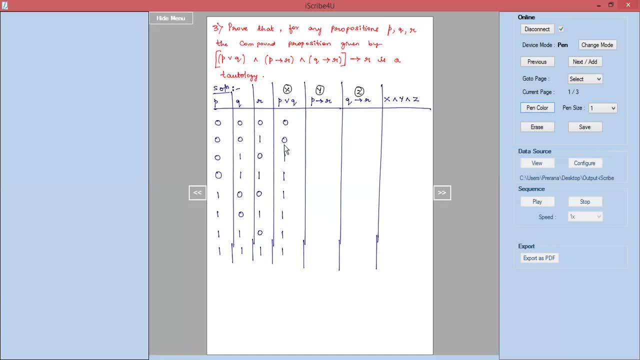 or the truth value of both p and q are false, then p or q is false. rest all cases. it is true same thing we have written. next we have p conditional r. first, in the third column you have to look into p conditional r is 0 only. 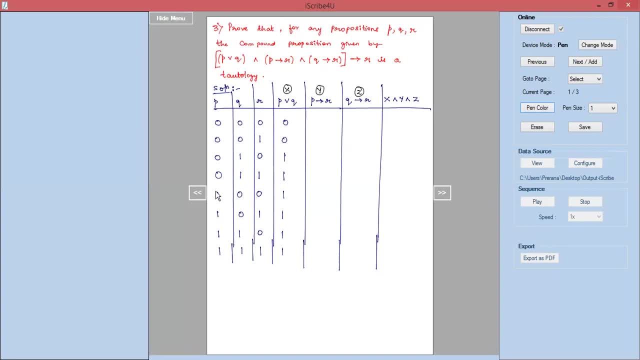 when p is true and r is false. p is true, r is false. one zero only when it is one zero resultant is zero. so one zero resultant is zero. again we have one more here: one zero p and r column you have to look into. so one zero resultant is zero. 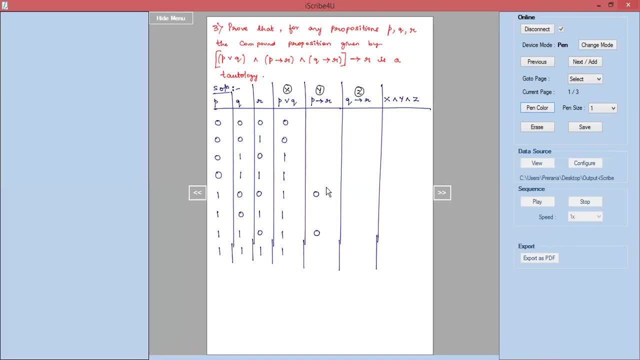 rest all cases. the resultant is one. rest all cases. there is that one. now we have to perform q conditional r. rest all cases. there is that one. now we have to perform q conditional r. second, in the third column we have to look into q conditional r again only when you have one zero. the resultant is zero. rest all cases. it is one. 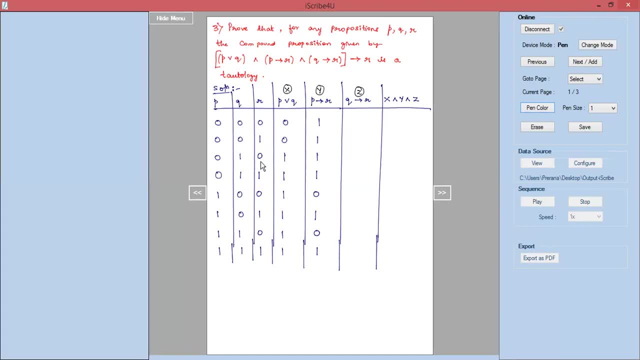 so third row, you have one zero. one zero is zero. then again, in the seventh row, you have 1, 0, 1, 0 or everything is 1, so rest, all cases are zero. rest, all cases are 1 and bottom row is zero. 1, 0 are perfect. then we have x and x. English values are even Ок. 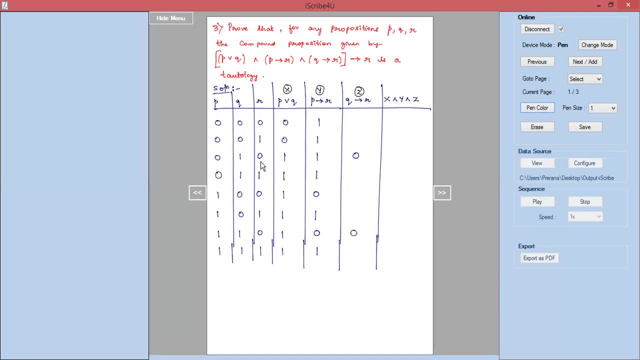 1th row, you have 1, 0 as 0.. That's all. now Rest. all cases will be 1.. All other cases are 1. only Now we are performing X and Y and Z For convenient. I had already taken. 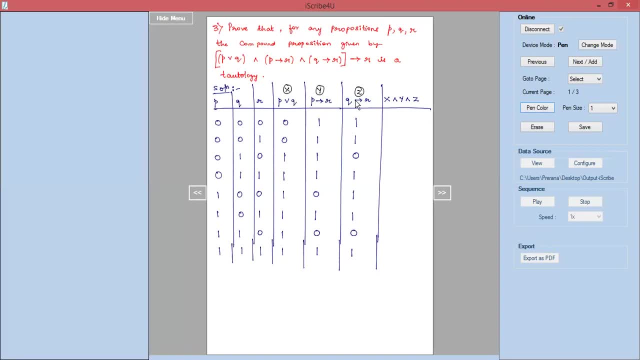 P or Q as X, P conditional R as Y, Q conditional R as Z. So now we are performing X and Y and Z. So AND between all the three means conjunction. When all the three are 1, the resultant is 1.. Rest, all cases, it is 0.. So, 4th row: we have all the values of X, Y, Z as 1.. So resultant: 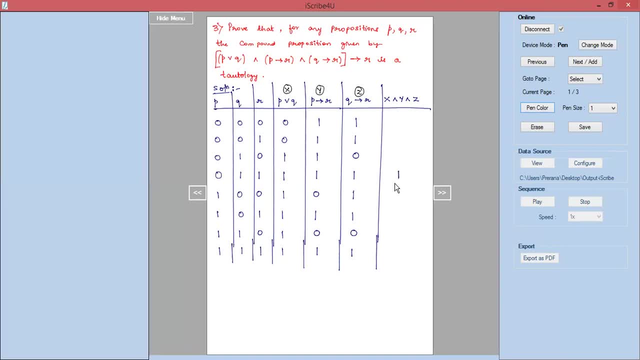 is 1.. Rest all cases it is 0.. So 4th row: we have all the values of X Y, Z as 1.. So resultant is 1. in the 4th row, Again, in the last row, we observe X Y, Z. all are 1., So resultant: 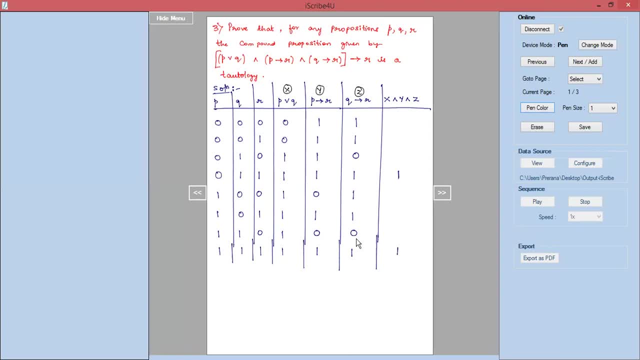 is 1.. If anyone of them have 0's- X and Y and Z- the resultant will be 0 only. So we fill 0's in the remaining places. So this is X and Y and Z. Now we have to perform. 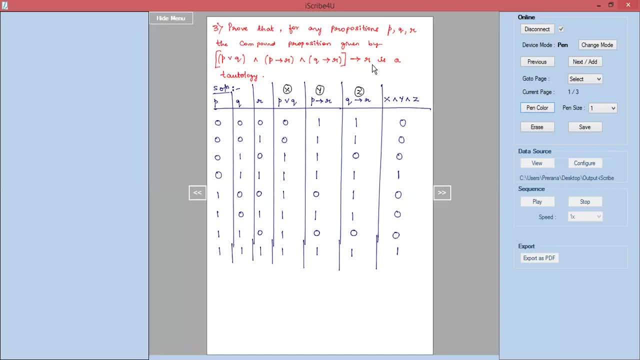 X and Y and Z, conditional R. Conditional R. We will perform that. I will just write down the answer here in the beside column, Just putting one column there. You try to manage it before only and put the columns accordingly. So here is my final answer. Answer. I am writing. 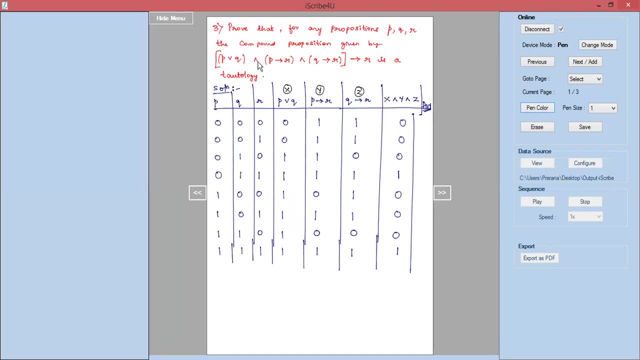 at the last column here. Answer: in the sense I have to prove this is a tautology node. So I am performing. What am I actually performing? I will write down here putting an arrow. So I will just write it in the other ink so that you can get differentiated. 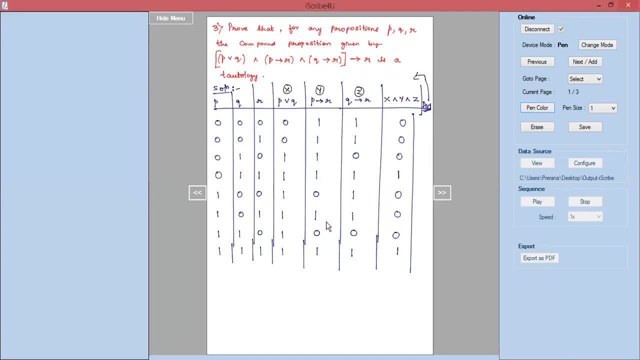 Okay, So what am I actually performing? is X and Y and Z conditional R? X and Y and Z conditional R? I am performing Correct, no? So what is the result? and then X and Y and Z conditional R, column Third column. you have to look, So you are reading the other way. 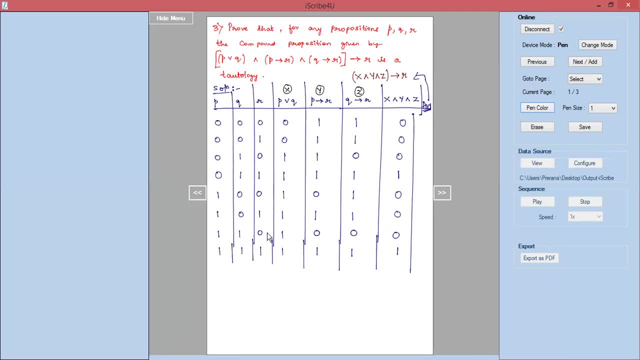 This column. you have to read it first, and then R column you have to read: And for conditional: only when you have 1, 0, resultant is 0. So I have to check whether I have 1, 0. So in this column it is 1. here The respective column of R has also 1. Again. 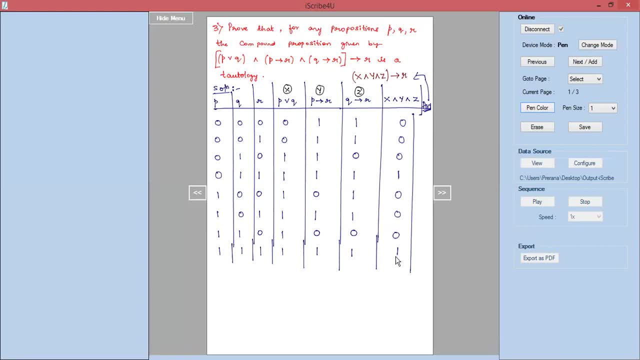 you have 1 here at the last, So respective column of R also has 1.. Only in the conditional. in the conditional, only when it is 1, 0, the resultant is 0. But we observe there are no 0 happening. So all the values will give you 1 itself. The resultant is 1 itself. 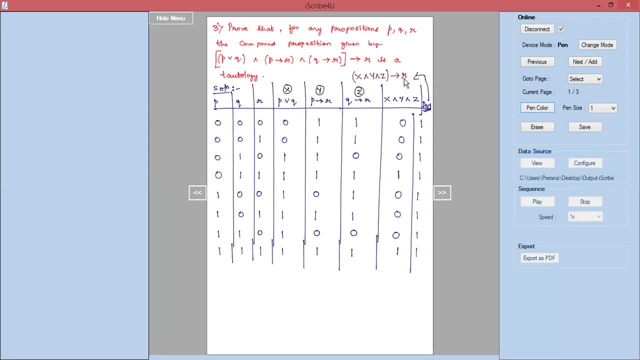 So we have proved that X and Y and Z conditional R has the truth values 1 in each of the compound propositions. So we can conclude that the required resultant is a tautology. So we can conclude Therefore: P over Q and P conditional R and Q conditional R, The whole conditional R is: 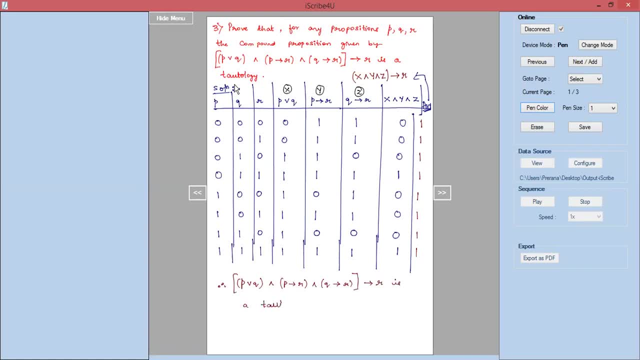 a tautology Is a tautology. Next Fourth one. Fourth one: Use truth tables. Use truth tables to verify. To verify Negation P and negation Q and R. You can write down appropriately: Or Q and R, or P and R is logically equivalent to R. Hope you can recall. This is the signal. 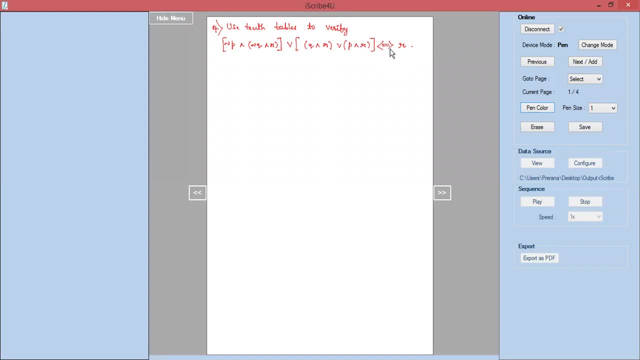 for logical equivalence. So definition of logical equivalence is that for each of the compound propositions, irrespective of the truth values, Whatever the truth values you have on the left hand part should be same as R. If I assume this as entire expression, as U and R as V, Then I have to prove that U is logically equivalent. 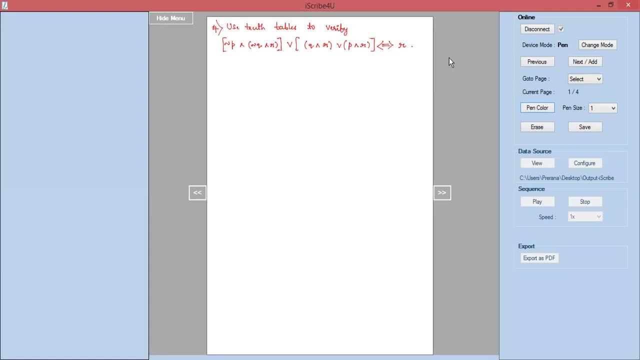 to V. They should have the same truth values. Then we can conclude that the entire expression in the left hand part is logically equivalent to R. Let us do the solution for the same. Let us do the solution for the same. I prepared this table so that we can have values now. So we have three compound propositions. 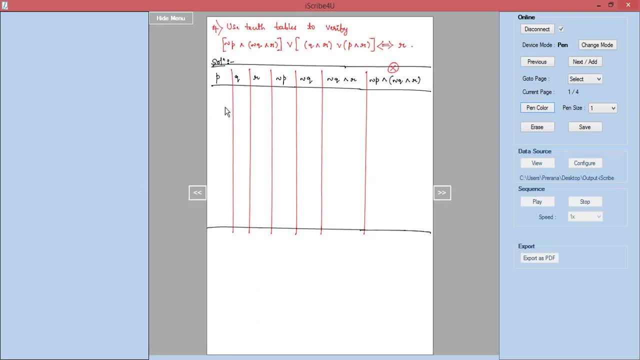 Three propositions, that is P Q R. So first three columns I prepared as P Q R. We observe in the first expression I have negation P, I have negation Q And I have negation Q and R. 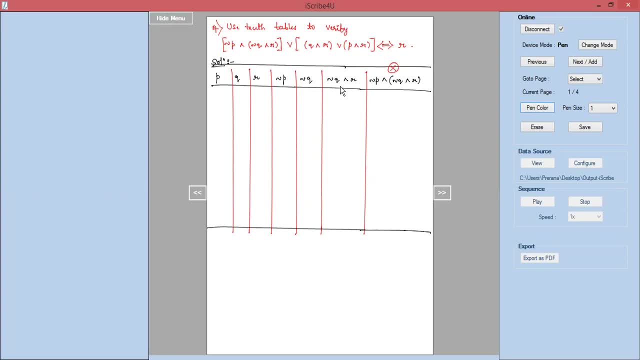 In a bracket, small bracket, we have negation Q and R. In a bracket- small bracket, we have negation Q and R. Then finally the first big bracket says that it is negation P and negation Q and R. So I have just denoted, for convenience, as X. Okay, Now we will fill in. 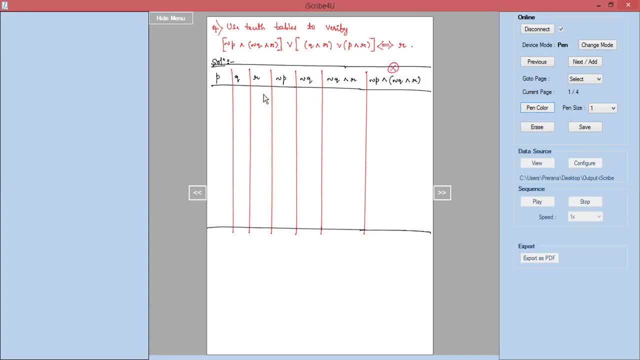 the values of P Q R. P Q R takes the values. They take the values as 0, 0, 0, 0, 0, 1, 0, 1, 0, etc. We will fill them first now. 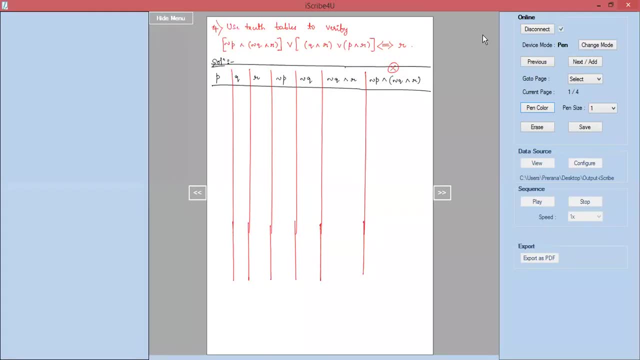 Okay, Okay. So we have 0, 0, 0, 0, 0, 1, 0, 1, 0.. Then we have 0, 1, 1, then 1, 0, 0, 1, 0, 1, 1,. 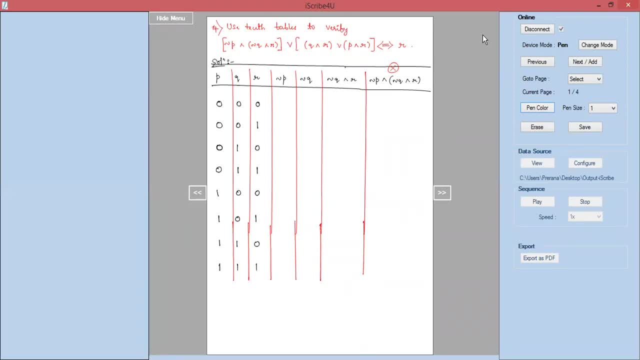 and finally 1, 1, 1.. We will fill the table negation P. So negation P means if you have 0, result will be D1. So like that we will fill. Then we have negation Q, Looking into Q column negated. So we have 1, 1, 0, 0, 1, 1, 0, 0. 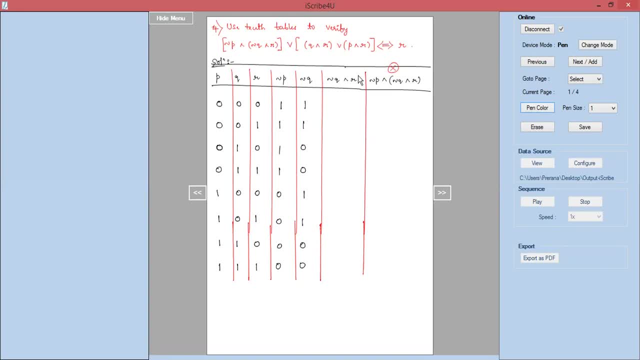 Okay, Okay, Okay. Next column will be negation Q and R. So next column I have to perform negation Q and R. So negation Q is this column, just now, what we obtained, and with R, So only when both are 1, resultant is 1.. So second row is 1 for me, And then we have that's all Okay. 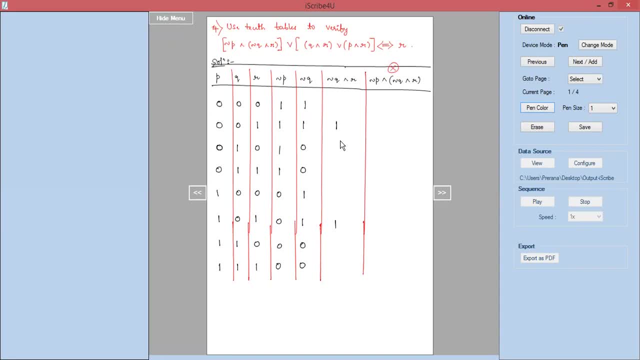 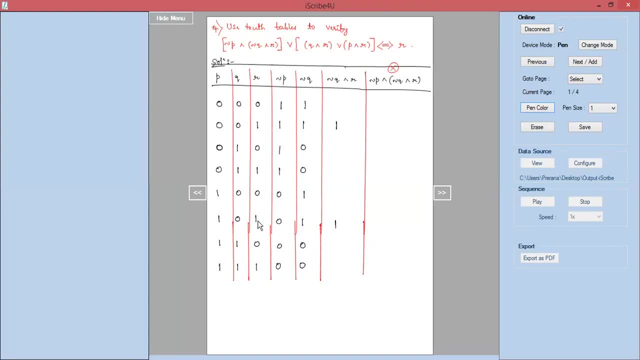 resultant is 1.. So rest all are filled with 0s. now, Rest all are filled with 0s. Next we have negation P AND Negation Q AND R. Negation Q AND R is just now what we obtained, that column We have. 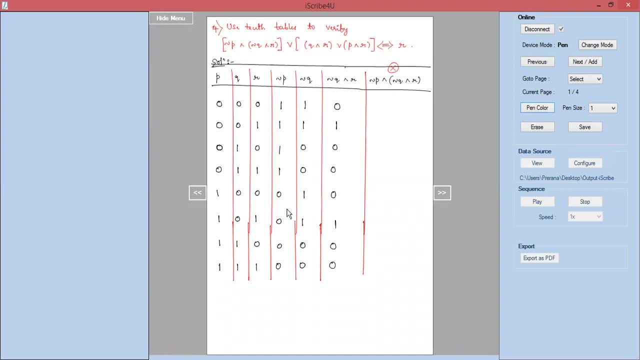 to do, AND with negation P. Negation P we have obtained already. So when there is both 1, you have to look into It is 4th column and the 6th column, I am looking Right. When both are 1, resultant is 1.. Rest all are 0s. Rest all are 0s. So only we observe that. the second, 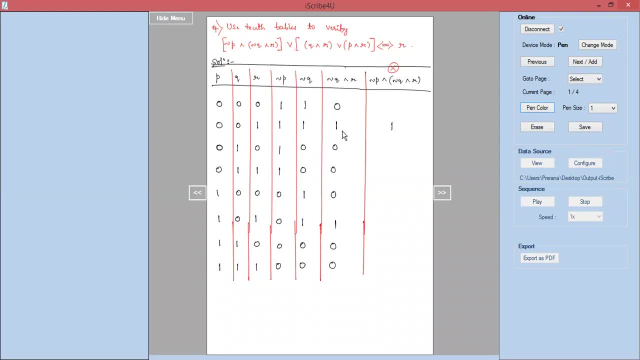 row is 1.. Second row resultant is 1.. All others are 0s. Rest: all are 0s. So only we observe that the second row is 1.. Second row resultant is 1.. All others are 0s. Rest. all are 0s. So only we observe that the second row is 1.. All others are 0s, Rest all are 0s. So only we observe that the second row is 1.. All others are 0s, Rest all are 0s. So this: 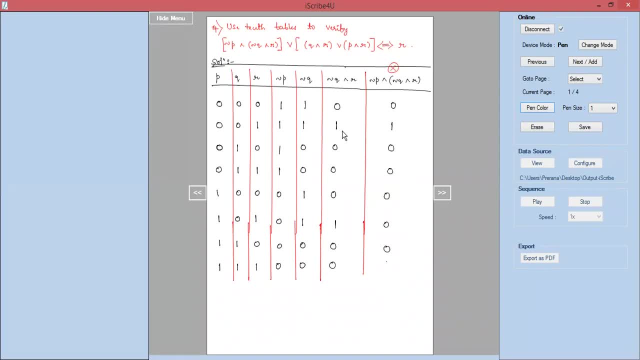 is the resultant, what we obtained now. Now, this is just X corals. I have to do still Q AND R or T AND R, Since I have a lack of columns required here, so I will just move on to the next page. You can just continue in the same table. Try to do it in one particular. 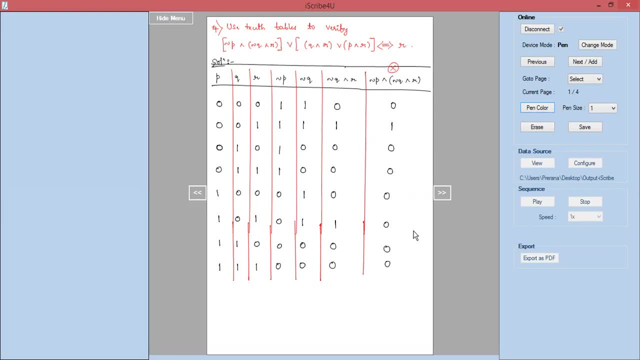 row wise, But at a stretch, if you are able to complete, you will have a better clarity. Now I prepared this table so that it will be convenient for us to look into and proceed. I have to next proceed doing Q&R, P&R and OR between them. 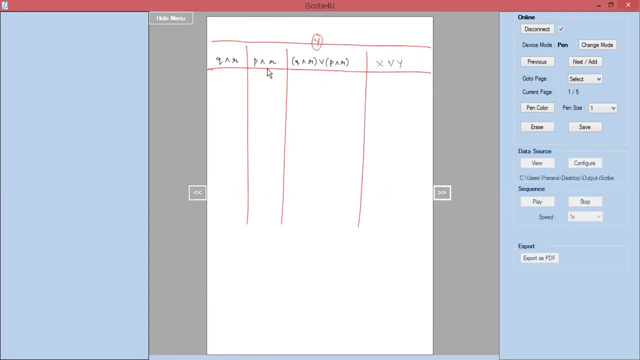 Correct, Same thing. I have prepared Q&R, P&R and there is an OR between them, which I called it for convenient as Y- Y. So this was our second big bracket in the left-hand bar. So now I have to perform X or Y at last. 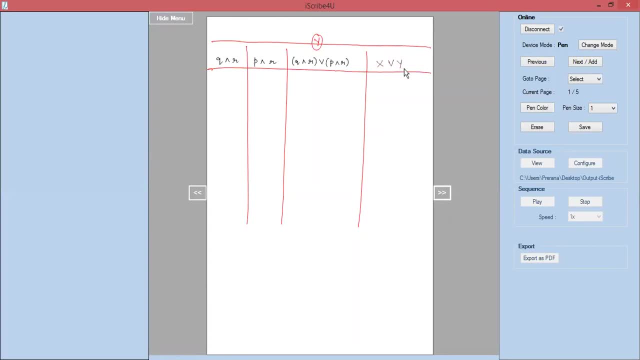 So performing X or Y at last. right. What to show? X or Y has the same truth values as OR, OR column, That is. then we will be proving that it is logically equivalent Right now. So we will now perform Q&R, P&R. 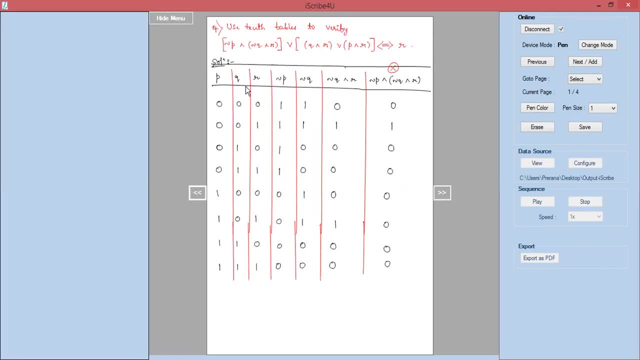 Since we are all now familiar with AND between the two propositions, we will just write down the values. So Q&R has the values 0, 0, 0, 1, 0, 0, 0, 1.. 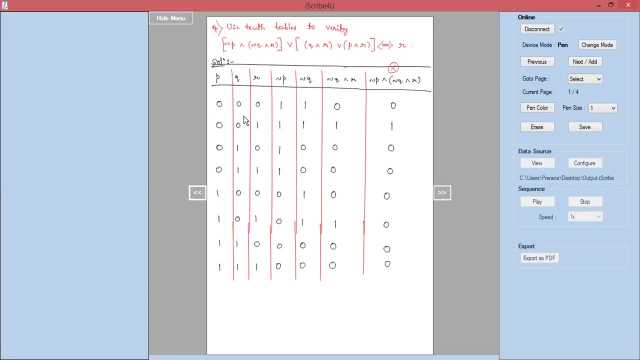 Q&R has these values We are all familiar with AND between them. So only So the resultant, and both are 1.. The resultant is 1.. Again, the last row we can observe. both are 1.. So that is why resultant is 1.. 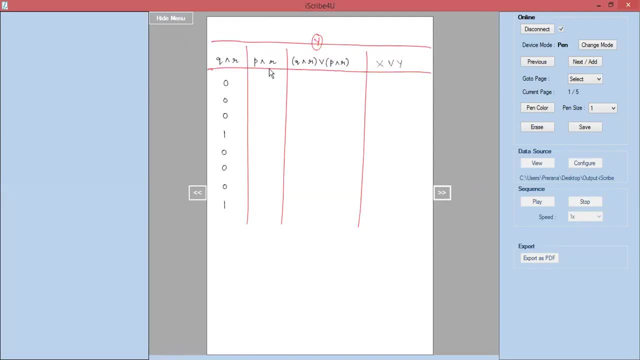 So rest all are filled with 0s. Similarly P&R. we have to do P&R, So we have both being 1 only in the 6th row and the 8th row P&R. So that is why 6th row and 8th row will have 1.. 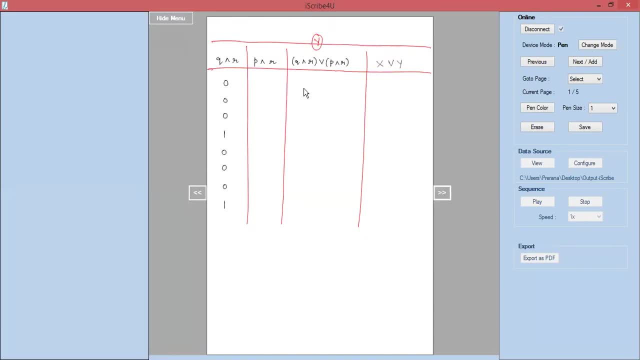 Rest all will be filled by 0s. 6th row as well as 8th row. Rest all will be filled by 0s. So this is for P&R. Now we have to perform Q&R or P&R Means, OR between these two. 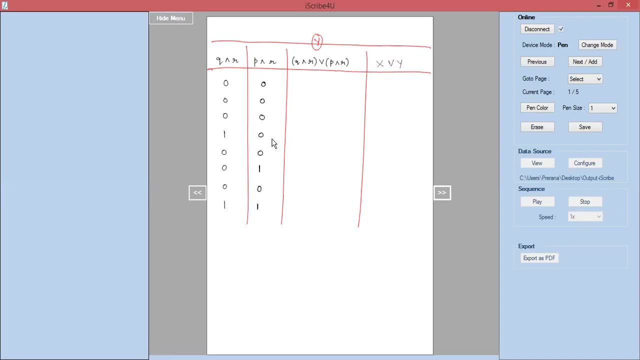 OR between these two means: if any one of the truth value has 1,, then the resultant is 1.. Correct, So 4th row resultant is 1.. 6th row resultant is 1.. 8th row resultant is 1.. 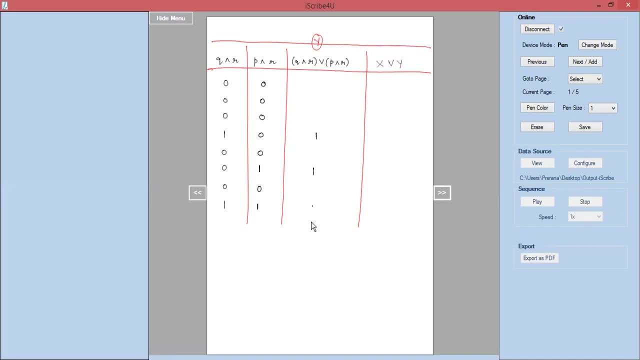 4th row, 6th row and the 8th row. resultant is 1.. Rest all are 0s. Rest all are 0s. Now we have to perform X or Y. We have X in the previous column OR between Y. 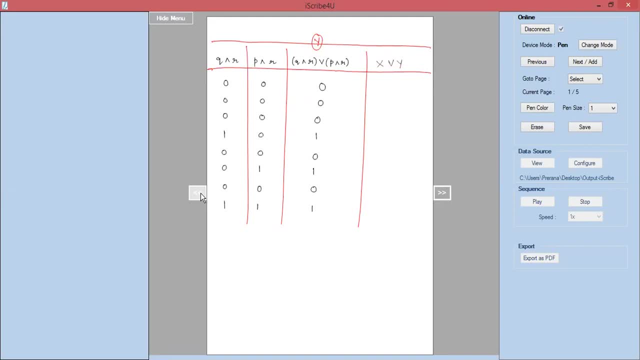 Y is this column for this. So what does X or Y say? X or Y means if any one of them is 1 in that row, then the value is resultant will be 1.. So 2nd row, there is a 1.. 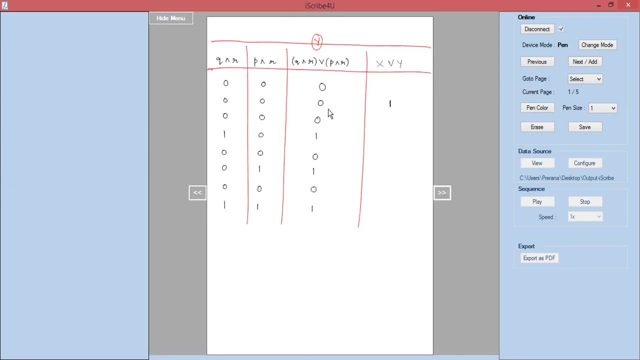 So 1 or 0 gives us 1.. 2nd row will be 1.. Then we have 4th row, 6th row and 8th row as 1.. 4th, 6th and 8th row as 1.. 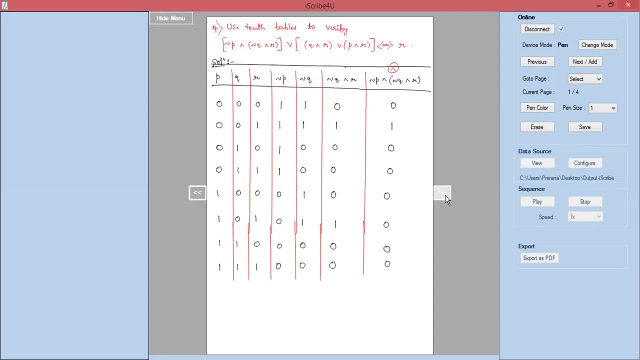 When you do OR with anything that is 0 or 1,, your resultant will be 1 itself. So you have 4th row 1.. 6th row 1. And the 8th row 1.. Now rest: all will be filled by 0s. 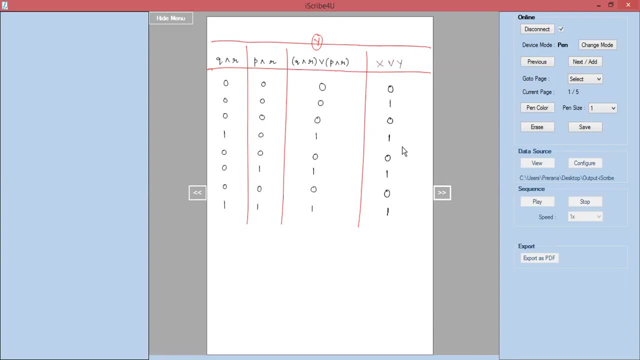 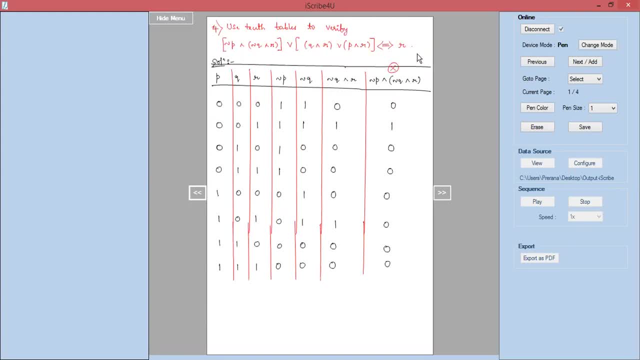 So right-hand side, you have to prove it is logically equivalent to R. Let us check the R column. You have R column as 0, 1, 0, 1, 0, 1.. And it was the same thing with X or Y. 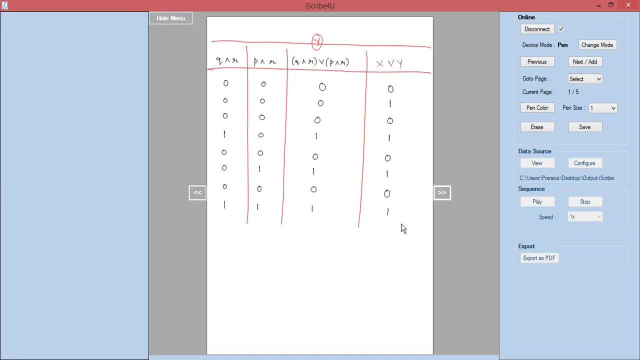 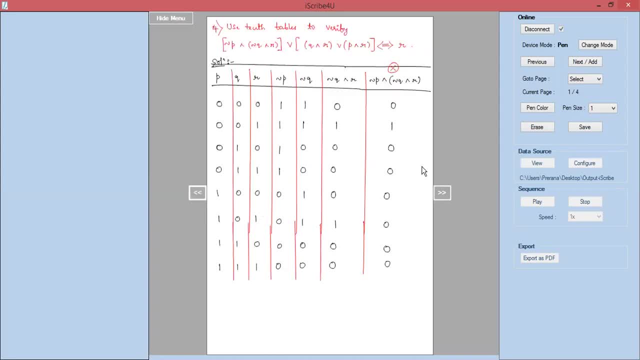 Third column is R 4,, 5,, 6,, 7,, 8,, 9,, 10, 11.. This is the 11th column resultant. So we are observing from columns 3 and 11.. The truth values. 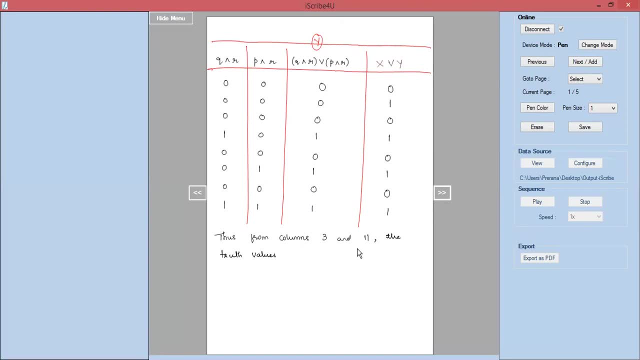 The truth values are same for all possible truth values of R, So for all possible truth values of P, Q, R. we observe the columns 3 and 11 are same, So that is why we can conclude: the left-hand part is logically equivalent to the R. 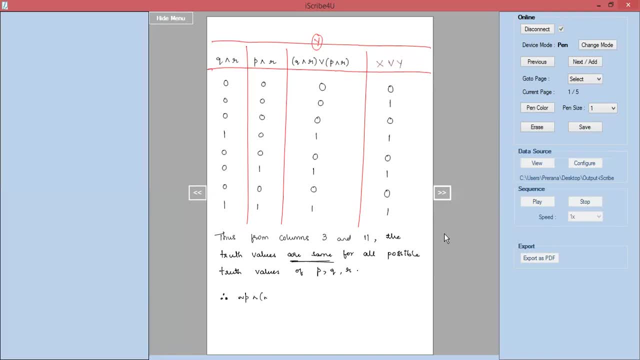 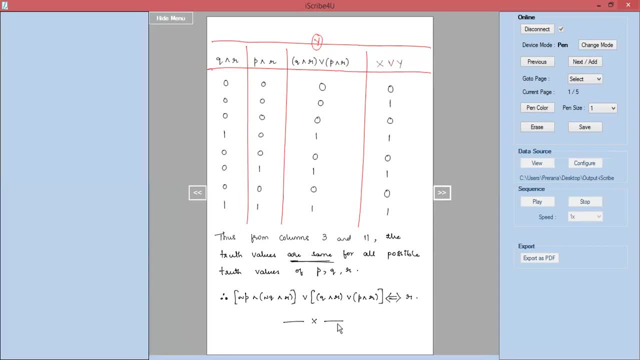 So I will just give one or two problem practice questions which will help you to get more idea about these two tables. Try doing them. So, in that I would like to give first one Practice questions, First one. I will give the resultant to be proved as a tau tonic. 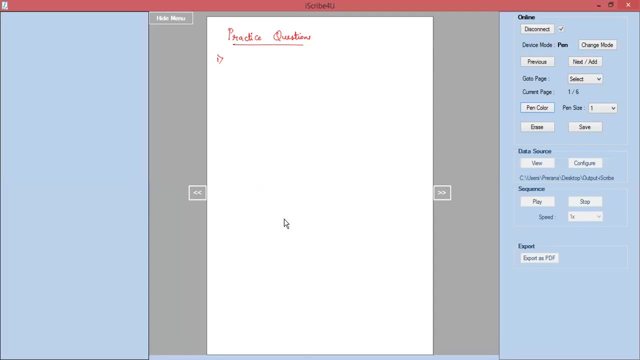 So prove that. Do that. Do that For any propositions P Q R. For any propositions P Q R. The compound proposition P or Q, conditional R, Biconditional Negation, R, conditional Negation of P or Q is a tautology. 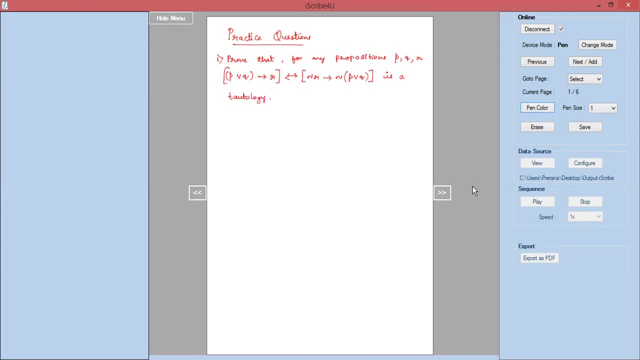 So you are familiar. what is a tautology? The final resultant, what is the compound proposition that you are proving? This entire expression should be a: Should have the truth values 1.. Should have the truth values 1.. So this is biconditional for us. 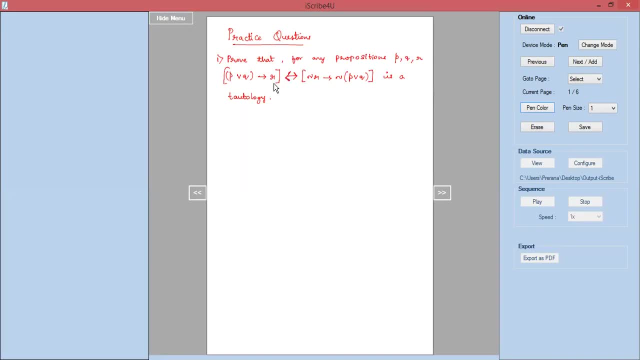 Biconditional here in the middle. So So you have to perform this and prove that it is a tautology. Second one: Prove that for any three propositions P Q R. For any three propositions P Q R. 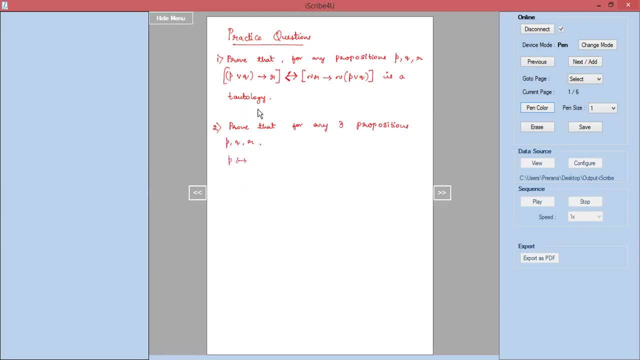 You have to prove the resultant P Q R, P Q R, P biconditional Q And Q biconditional R And R bicondition P. This entire expression is logically equivalent to: